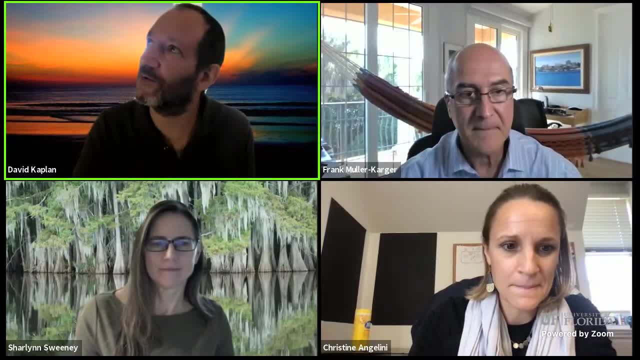 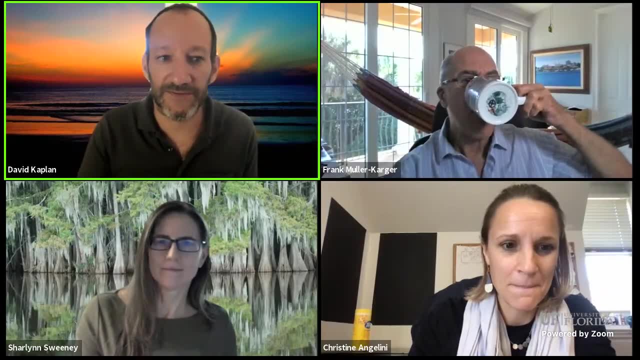 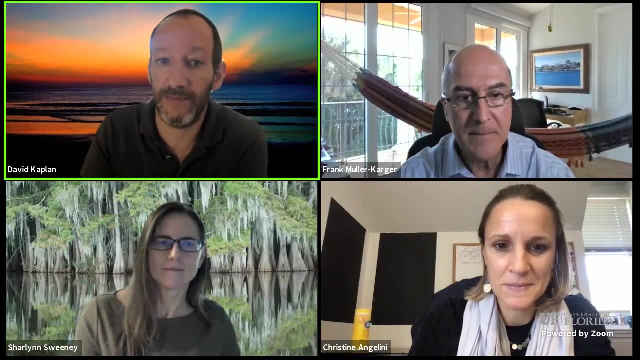 Welcome back everyone. It's our wetland, watersheds and water, wetland and watershed seminar. It is fall 2021, October 27th. Today, we are fortunate enough to have with us Dr Frank Muller-Karger. Dr Muller-Karger is a professor of biological oceanography at the College of Marine Science at USF University of South Florida. 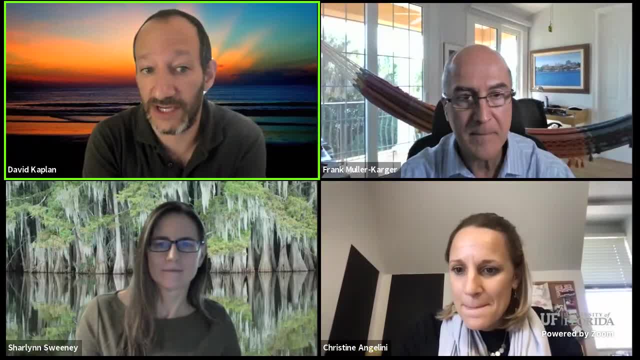 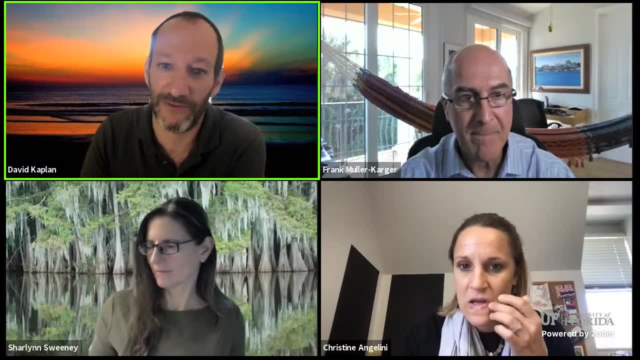 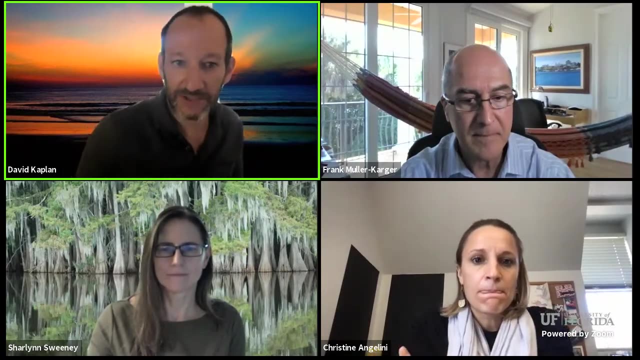 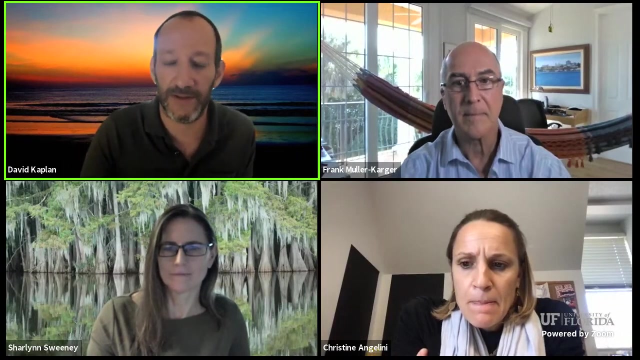 Dr Muller-Karger conducts research on how marine ecosystems change in time, using both traditional oceanographic methods- going, you know, out to the sea and measuring things all throughout the water column and at the water surface- but as well as using satellite remote sensing, so sensors, to study changes in water quality, production, biodiversity, and much of his work is focused on improving our ability to measure and observe phytoplankton using remote sensing. 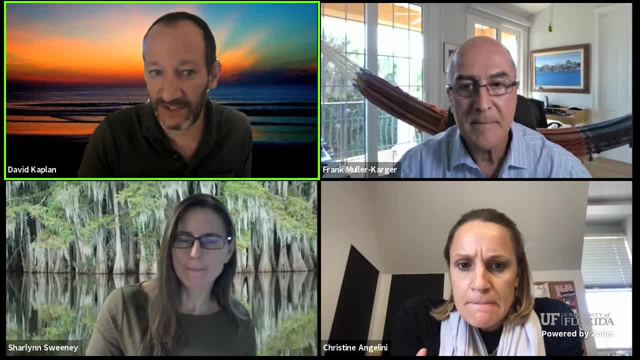 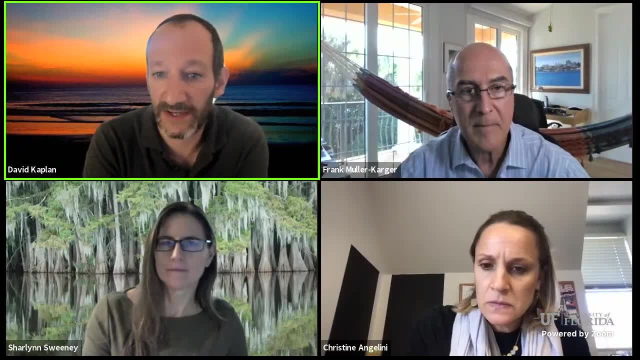 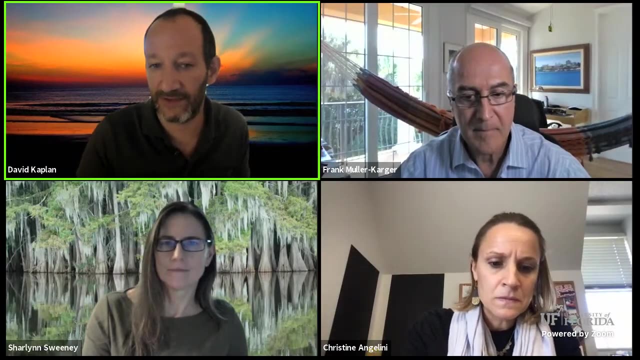 Beyond research, Dr Muller-Karger has a keen interest in linking science and education and particularly addressing the problem of underrepresentation of minorities in scientific research. So he's worked hand in hand with K-12 teachers and students to showcase new technologies, highlight the importance of oceans in our daily lives and to improve sort of the access of underrepresented minorities into science. 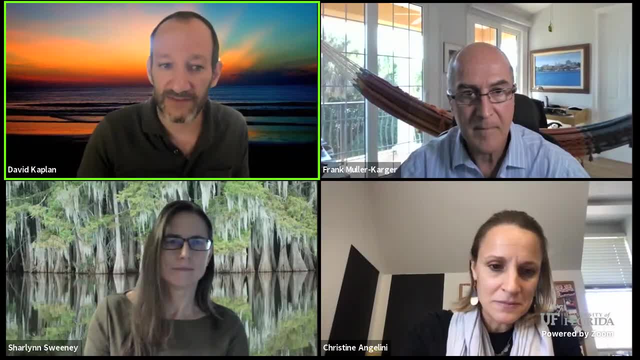 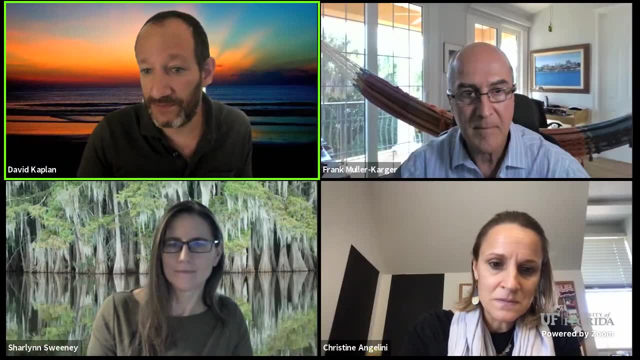 Dr Muller-Karger has a BS, MS and PhD degrees in marine science and as well as a master's degree in management. He's co-authored over 120 scientific publications and served on the US Commission on Ocean Policy, As well as the Dean of the School for Marine Sciences and Technology at UMass Dartmouth. 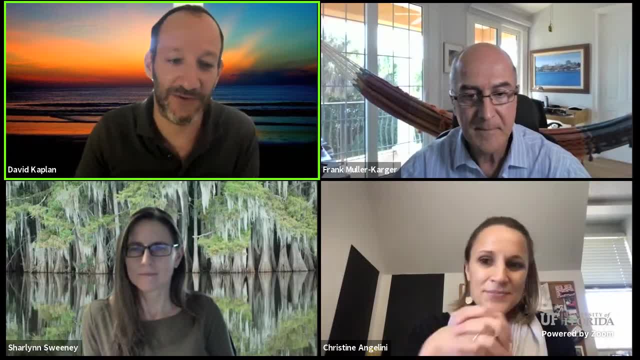 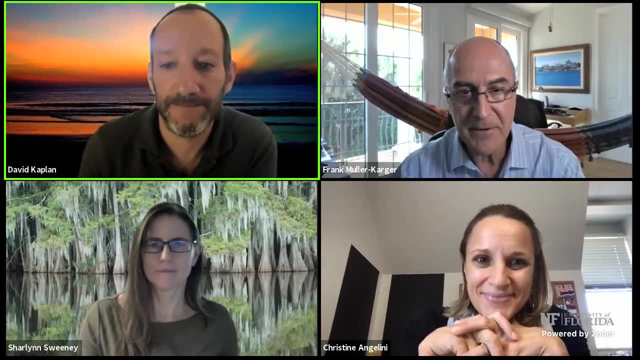 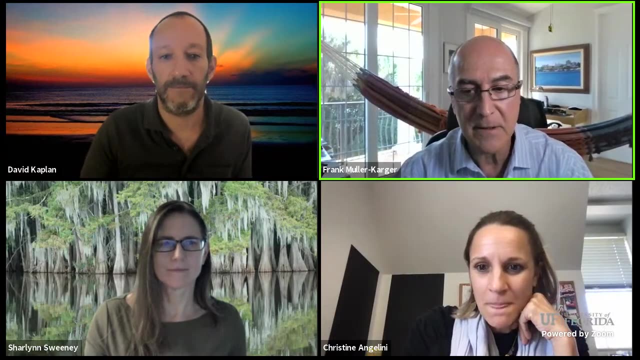 So, without further ado, Frank, please you may go ahead. The floor is yours. Thank you, Can you hear me okay? Yep, sounds good, Great. Thank you for the opportunity to be with you. I'm going to talk to you a little bit about some programs that we're organizing nationally, working with several agencies, but also internationally. 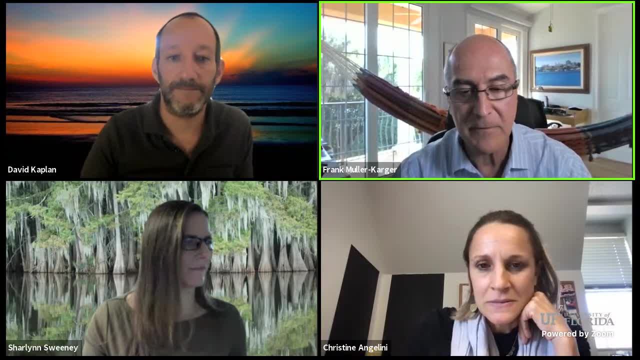 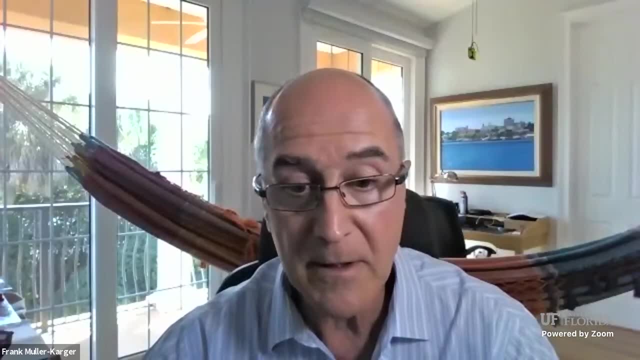 and how that evolves over time. I'll give you some of the results that we have for some of the things that we're doing locally in the Florida Keys, but also nationally. So I'm going to share my screen and I hope you can see that. 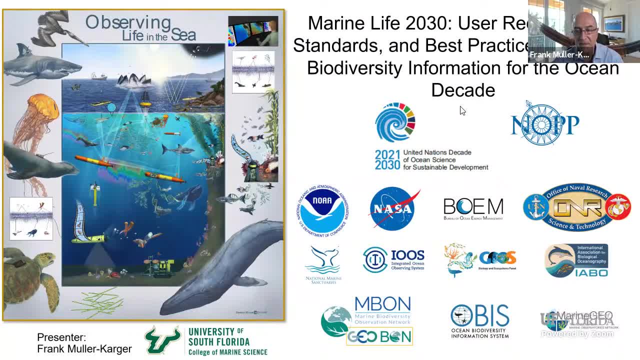 So, if you can give me a, Looks perfect. yeah, Okay, great. So there's a busy screen of logos here because we are working with so many people And it is It's very hard to see- Yeah, It's very hard to acknowledge everybody that we're working with. 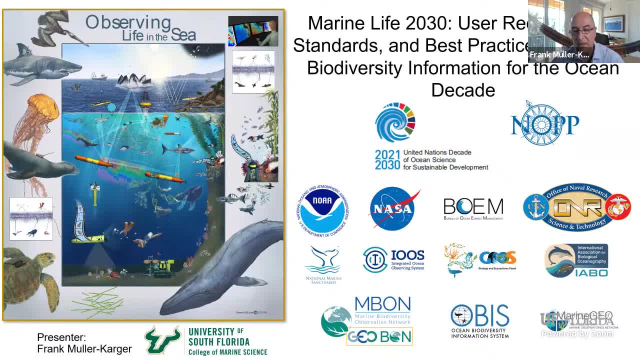 The work that I'm going to present to you largely is sponsored by NOAA and NASA. It is also a larger program that is sponsored by the Bureau of Ocean Energy Management and the US Navy. There's many, many other groups, And they're all coordinated nationally through something called the National Ocean Partnership Program. 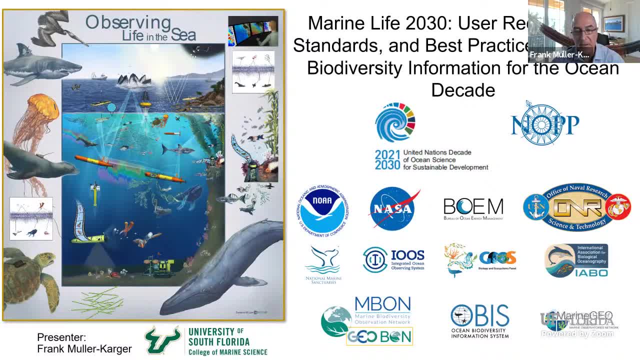 which I hope you take a look at at some point, because it's a way that US agencies and the- the administration at the federal level- used to share funds, And so there's a- I don't want to go on a tangent, but it's a very important program that we have in the US. 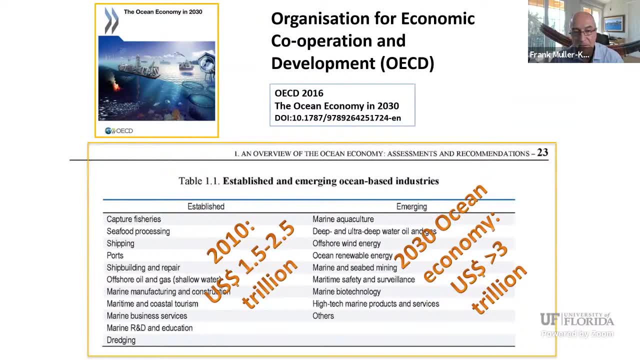 So one of the reasons that I want to talk to you about this is because everybody talks about this blue economy and there's a lot of buzz around the blue economy, especially, one of the people that that really pushes this concept is Rick Spinrad, who's now the head of NOAA. 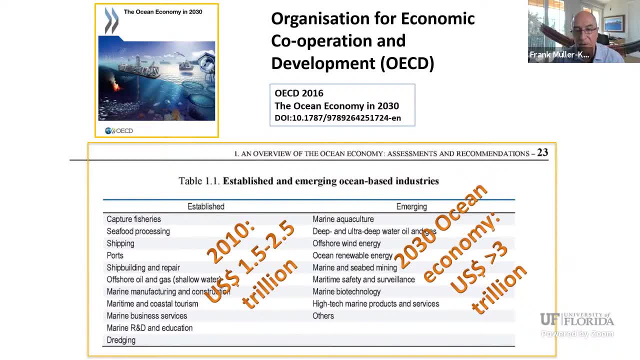 And so this has been. This is a concept that has been brewing for, you know, 10,, 15 years already, And it is the idea that there's a lot of jobs and a lot of economic benefit that is derived directly from the ocean. 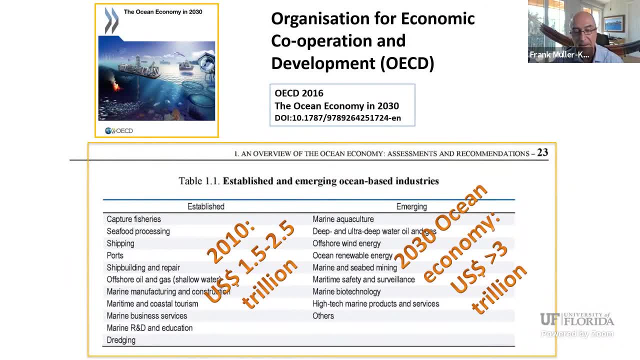 But also there's a cloud of other activities that are related to that, And if you count that, it's in the order of $1 to $2 trillion globally And that it's expected to grow. Now the thing is that we cannot just expect that this growth can be sustained. 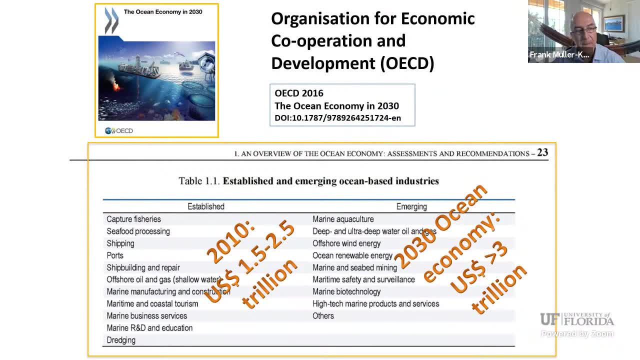 if we don't pay attention to how we normally exploit things in the ocean or how we use the coast. You know there's a lot of development and industry that unfortunately doesn't lead to a sustained economy because it just drives resources into the ground. 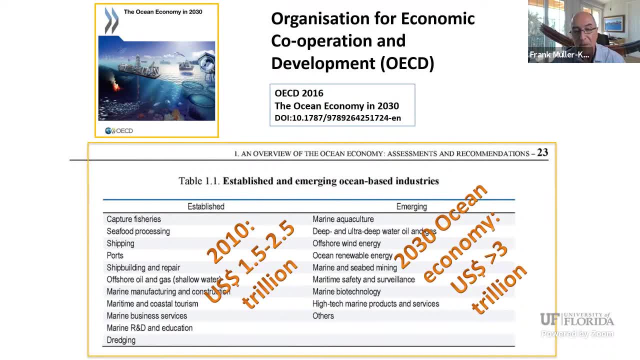 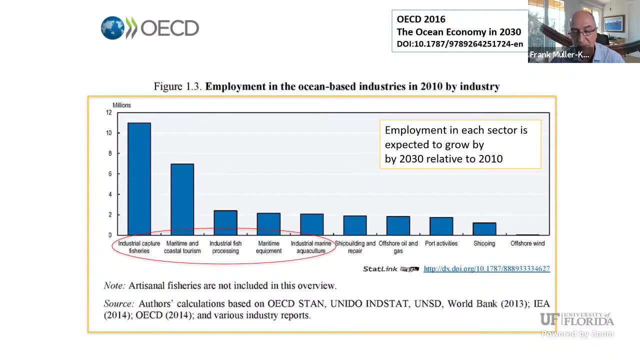 So the question is: how do we can sustain growth, produce more jobs and yet conserve the environment in a way that is beneficial to everybody, today and in the future? All of these jobs and all these industries that you can think of, and much of the blue economy, has something to do with life. 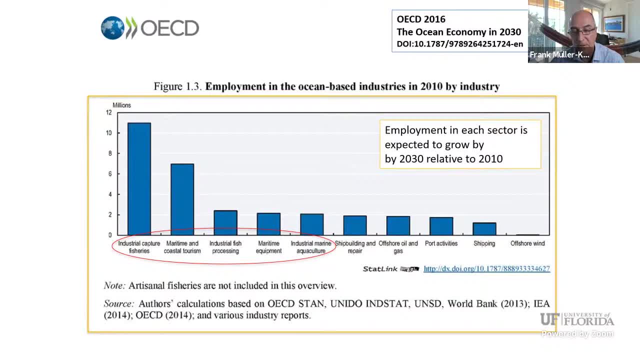 Either it's because you're fishing directly, recreationally or commercially, or you're doing agriculture, or you're doing navigation, or you're installing something in a coastal zone, some structure or whatever, Or some platform to drill or extract some resource from the bottom of the ocean. 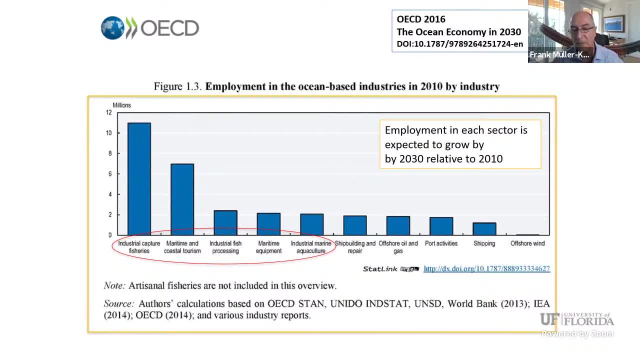 It all has to do with life, because you have an impact, And so either you have to do an impact statement or you have to preserve some other resource, And there's always some way. it always comes back to an invasive species or your destruction of habitat. 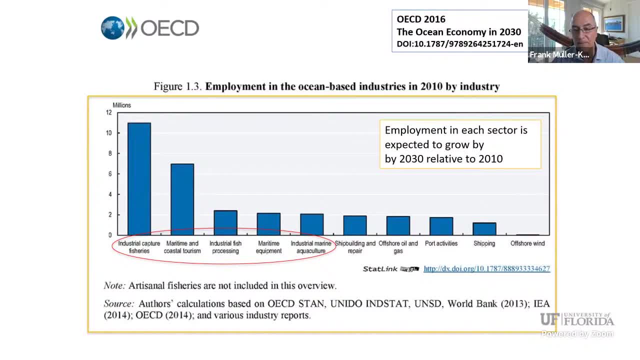 So the question is: how do we quantify what we're doing so that we know and manage these human activities? And so it's really about the human activity. How do we organize these human activities better so we can sustain this economy? So this is the idea where a lot of people have talked about this for many, many years. 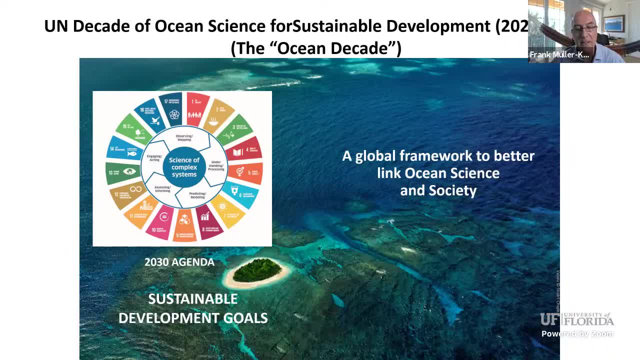 But one of the newest things is this sustainable development goal, or Agenda 2030.. And there's 17 goals. They're all really related to each other. There's no, not one that is really disconnected from the others, But people try to focus on individual ones. 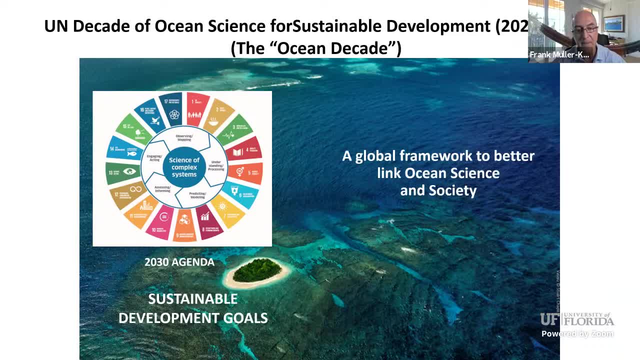 And so for the ocean, if you want to think about it that way, The Sustainable Development Goal 14, they kind of shortened the name to Life Below Water, but there's really anything that is related to the marine environment and how it links to all these other goals. 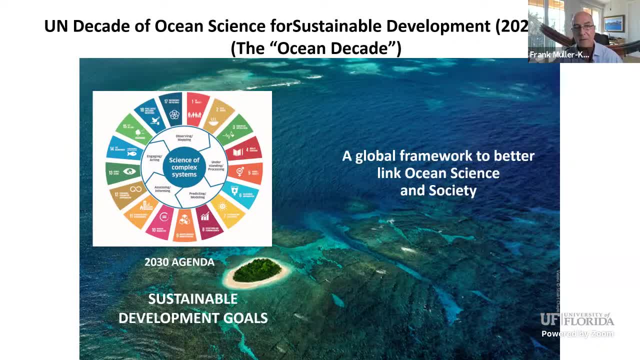 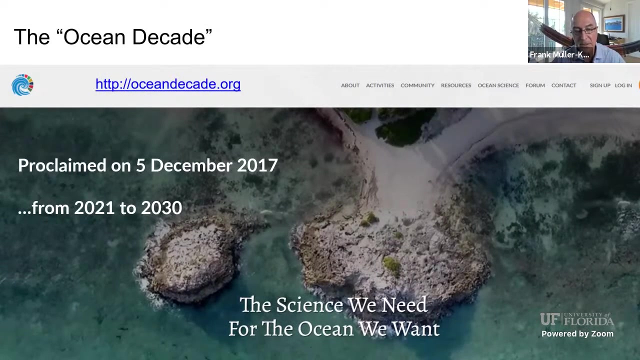 So that is SDG 14, and the United Nations worked with a lot of people to try to see how do you highlight what's going on in the ocean and develop a good framework for the economy and sustaining jobs? And so, leading up to 2017, they had a process to design this Ocean Decade or the UN Decade. 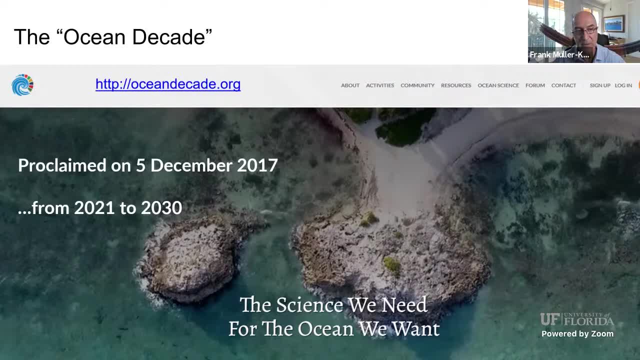 of Ocean Science for Sustainable Development, and so everybody shortens it to the Ocean Decade, which is more about sustainable development than about science. but how do you link those two things? And so this is part of what I'm going to talk to you about today. 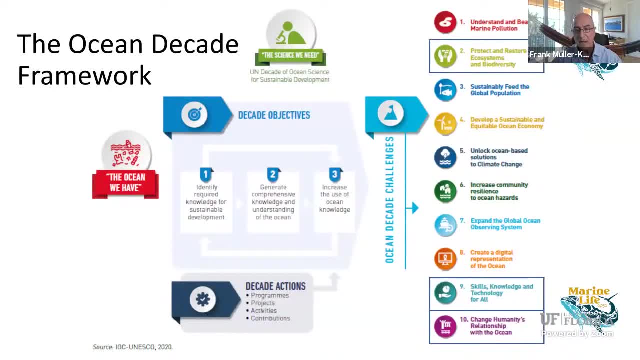 It's this Ocean Decade and how you can get involved. The Ocean Decade, basically, is driven by these challenges that you have on the right hand. There's 10 challenges. We- my group- is very involved in challenges 2,, 9, and 10, which is basically looking at. 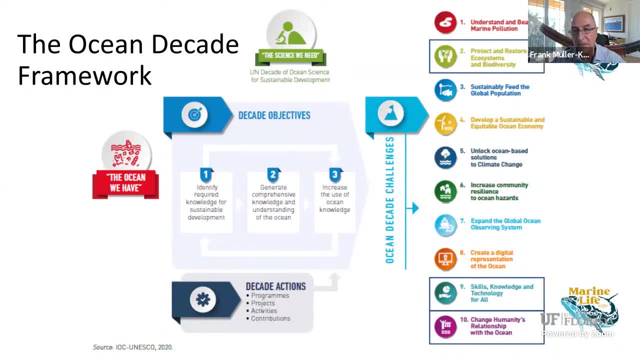 how ecosystems work and how do you use information about biodiversity? How do you develop the knowledge skills to not only collect data but use the data And then kind of have a public relations effort to try to bring the public more in tune or kind of broadening the audiences that we have to talk about the ocean? 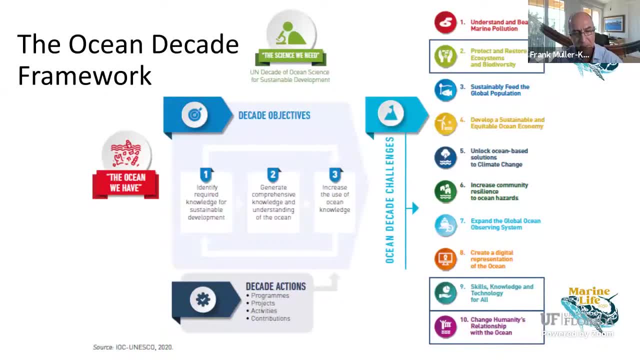 But if you look at it from the left hand side, the ocean we have. you know, the motto of the Ocean Decade is the ocean, the science to get to the ocean we want, from the ocean we have. So you have the decades. 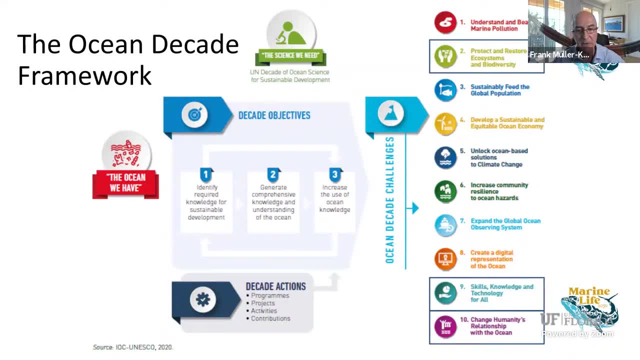 The Ocean Decade has these objectives. that is all about knowledge in the blue economy is intended to be a concept of of how do you use information to to drive the economy so you you can identify the knowledge, generate the knowledge and then use the knowledge. 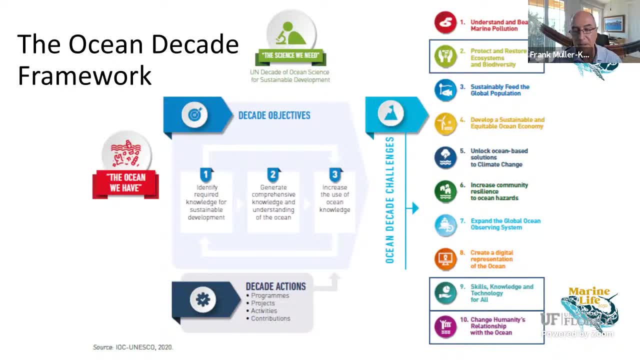 And those are the objectives of the decade. The way they do this is by trying to stand up what they call decade actions. The actions- there's a whole bunch of them. They're the highest level. It is what they call programs, which are kind of a framework that it can be global and scale long term and where you can fit a number of different projects under. 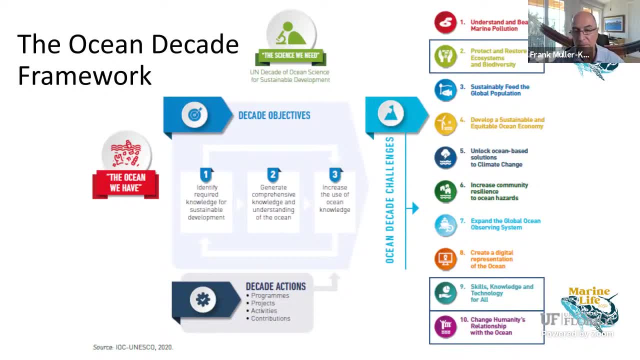 And then you have each project and have activities. activities would be more, more focused in a region or a series of webinars or or relatively, so it doesn't have to be global in scope and contributions are effectively how you, how you contribute in In a monetary 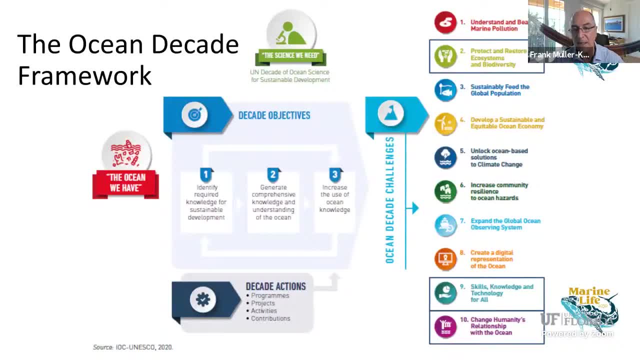 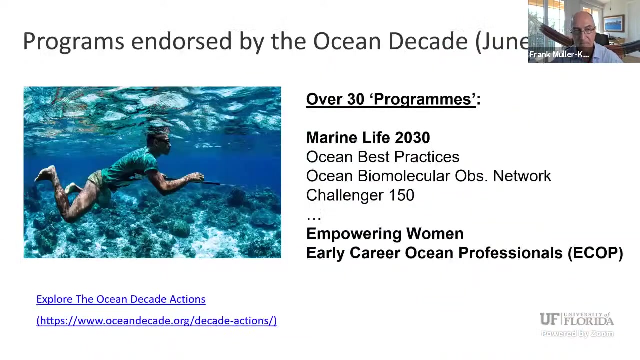 A monetary way or in a way that you can do an in kind contribution with people. So that way, these and these actions are in process now. they went through an announcement last year. they selected some programs and projects earlier this year and they announced them in June. and they now have on a new call that just came out about a week or two ago and I'll talk about that again. 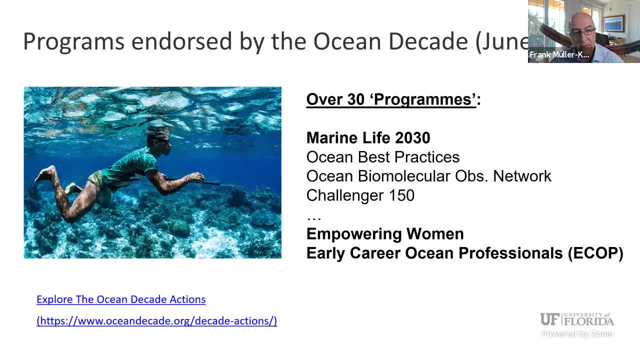 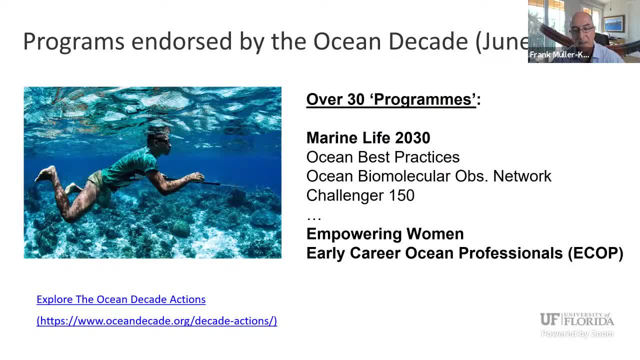 program or a project. They call it an endorsement, And the group that does that is called the Decade Coordinating Unit And that lives inside of something called the Intergovernmental Oceanographic Commission or IOC. The IOC is basically a program under UNESCO, So it's part of the United. 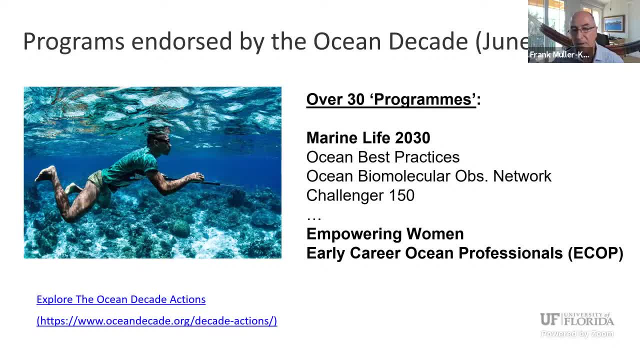 Nations. So what they did is they selected over 30 programs, And many of them are things that you may already know. There's one that's called Marine Life 2030, which we lead, And we want to invite you to that, But there are others in which we're involved in or not involved in, but we want to try. 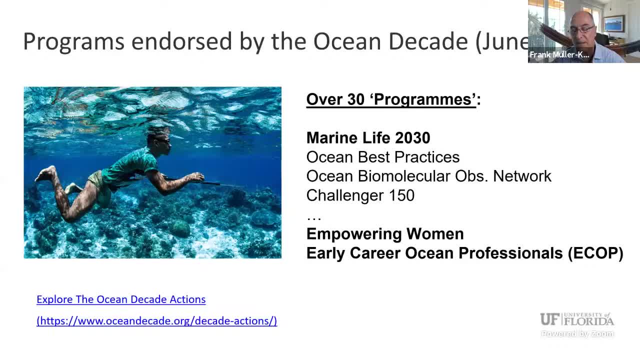 to coordinate with one, for example, on best practices. There's one on biomolecular: how do you stand up on a biomolecular observing network in the ocean? There's something called Challenger 150, which goes back to the Challenger expedition, and it deals with the deep ocean. There's also some that I think you need to be aware of that. 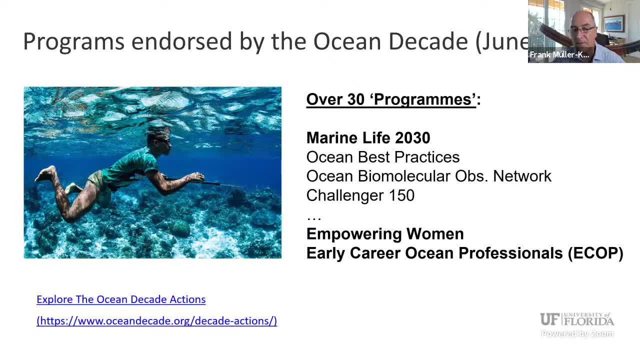 are trying to. the Decade is a very inclusive environment. They're trying to do things in terms of justice and equity and diversity, And so there's a program on empowering women and there's one on early career ocean professionals. So I encourage you to look those. 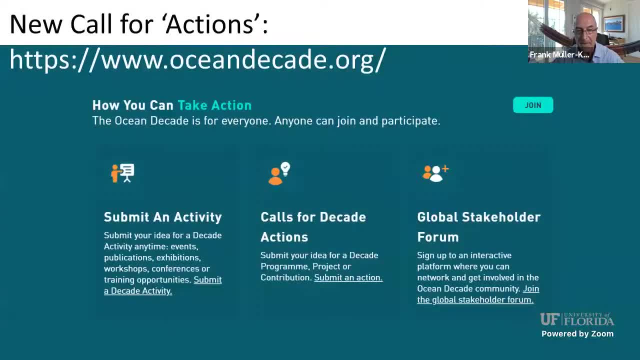 up and get engaged. The new call for actions released just a few days ago is: you can find it in this oceandecadeorg website And you can now submit proposals to join some of the existing programs, establish new programs or do something else like contribute some type of resource. So 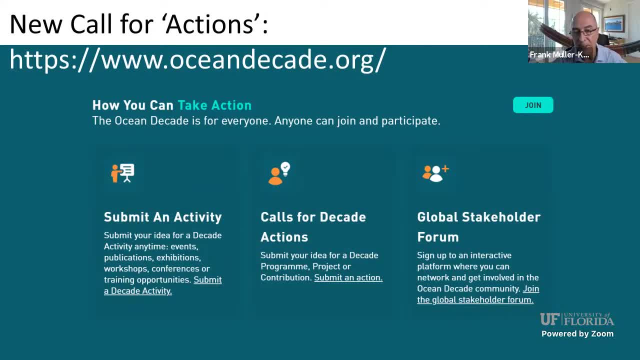 we're inviting people through this process And we're going to do that, And we're going to do that. We're also going to work with some projects at the US Governing Authority, at the Marine Life Project in the virtual неo, which is kind of artistic work, And from that point we're going. 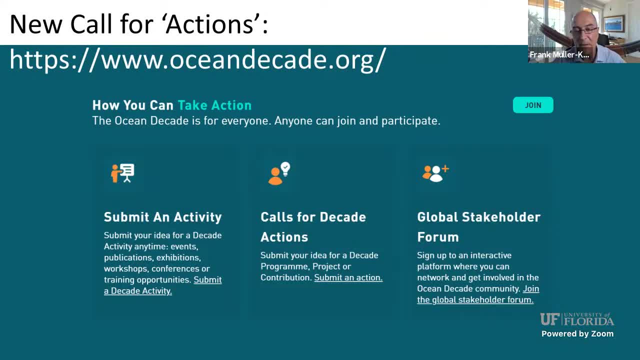 to looking at what is the best practices to contribute projects specifically to marine life 2030, and to join with other groups like the Biomolecular Ocean Observing Network or the best practices which we're trying to link together quite actively. So just kind of a time history of 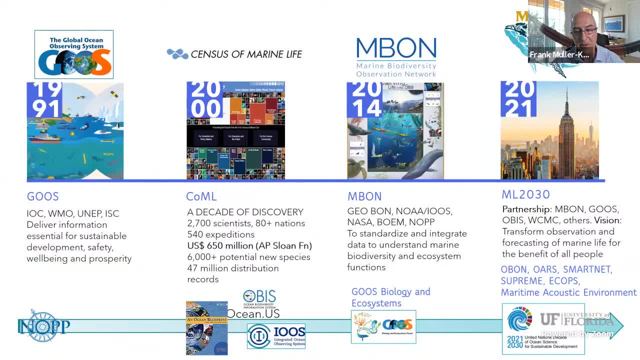 where we are today is if we go back to the early 1990s, And so you see that there's not a lot of time has gone by and a lot of things have happened, Yet there is an ongoing process in which we're. starting to find solutions for problems and strategies to be able to promote them. And that's definitely gonna happen in the future. And you know, and you know, in the future there's a lot of, There's a lot of things that still need to happen. 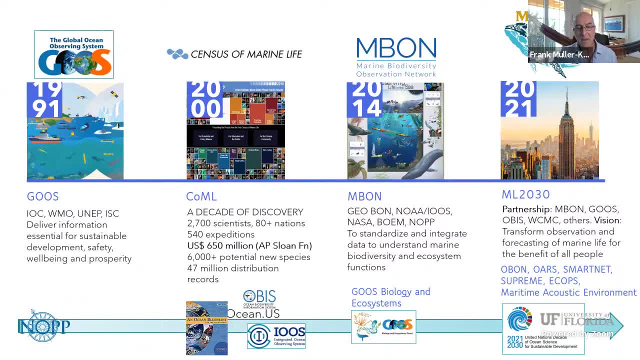 Way back in the early 1990s people were trying to organize the ocean observing community similar to what the weather community did 50, 60 years ago. So today you can find a lot of shared weather data: temperature, precipitation, you name it. 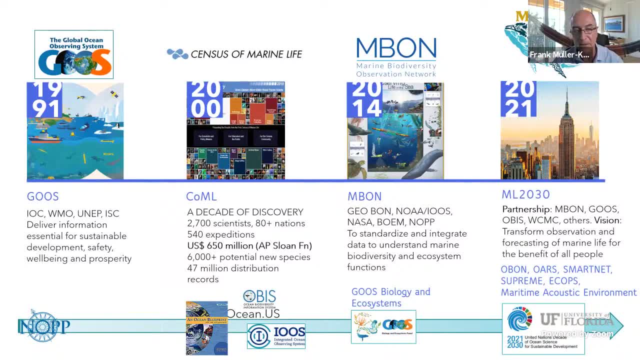 These are things that you need to forecast weather effectively around the world, And so the ocean community organized itself into something called the Global Ocean Observing System. that was sort of formalized and attached to the Intergovernmental Oceanographic Commission way back in 1991.. 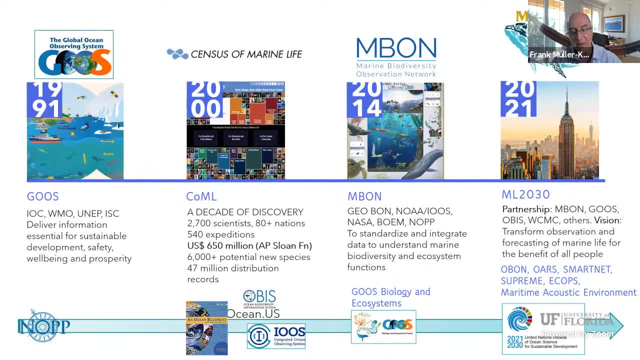 There were many things that were related to that that came out of that under the IOC. The IOC is a political body under UNESCO, so it has representations from member countries And typically these are countries, Countries that are coastal nations. Then in the 2000s timeframe a group decided that you know, goose is very important but it historically has been focused very much on physics and almost exclusively physics. 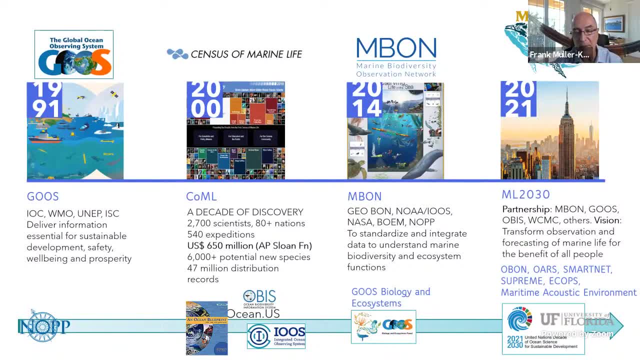 And slowly had been growing up by a geochemical effort because of the ocean acidification push. But even though there was a sense that we needed to measure biology, That wasn't really part of the of the formal operational activities that were being stood up under goose. 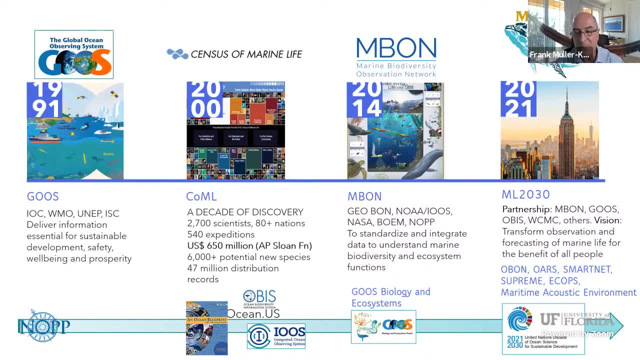 And if you think about goose and the US as a participant in goose under something called the Integrated Ocean Observing System or IUS, that's the US contribution to goose. And many different countries have their own regional, what they call a regional alliance around the world. 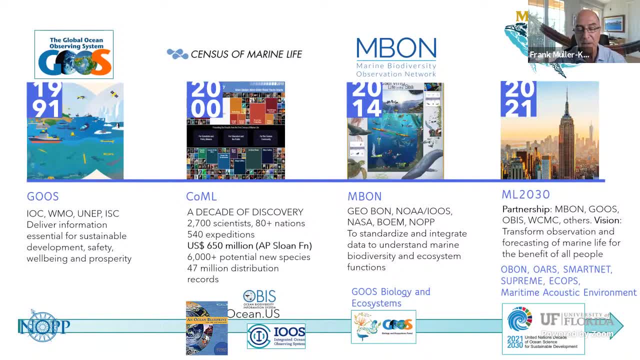 So people recognizing that The one thing that we were all trying to do we measure temperature, we measure weather, we measure all these physical things and the pH and chemistry of the ocean, because we think that it's going to have an impact on life. yet the last thing we were measuring is life, you know. so this is the, in part, because the technology drives what you can observe. there is this gap in how much or when, or how much information we have about the life in the sea, especially when we're talking about the ocean. 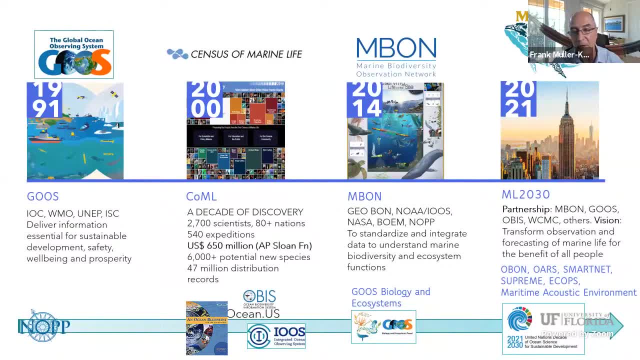 Right, Right, Right, Right, Right, Right, Right. What lives where? how much is there? what's the productivity? So these basic, fundamental biological observations are, even still today, not being collected properly And the end result is that we cannot forecast life the way that we can forecast weather or that we can forecast ocean currents. 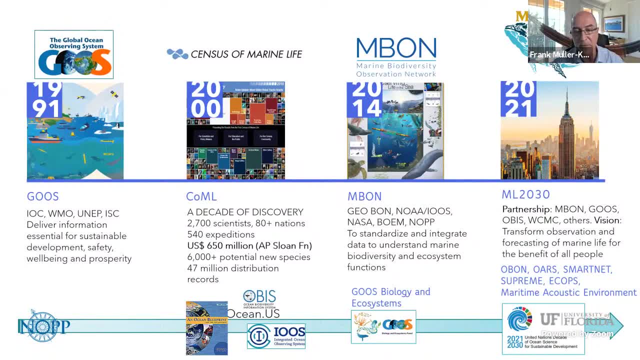 So we want to go in that direction and be able to forecast life, because we depend on our observations. So we want to go in that direction and be able to forecast weather, or that we can forecast ocean currents. So we want to go in that direction and be able to forecast weather, or that we can forecast ocean currents. 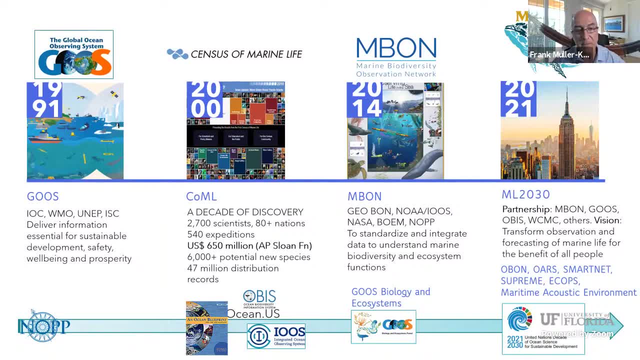 Our own life depends on how we manage this planet. So in the 2000s we stood up the census of marine life. that was privately funded- you know, $650 million- by the Sloan Foundation and it brought a tremendous attention internationally on detecting species where they live. 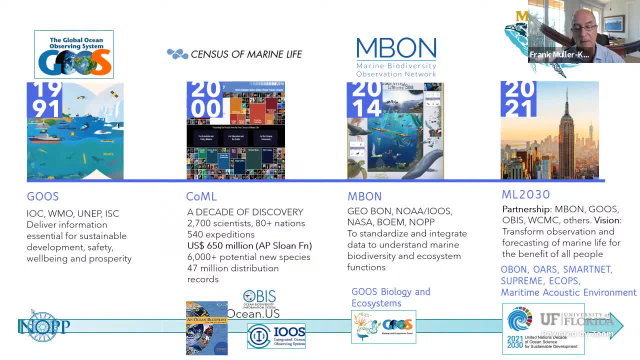 It's kind of more of a presence absence effort, just because we didn't have enough information even about what was living where. It's kind of more of a presence absence effort, just because we didn't have enough information even about what was living where. 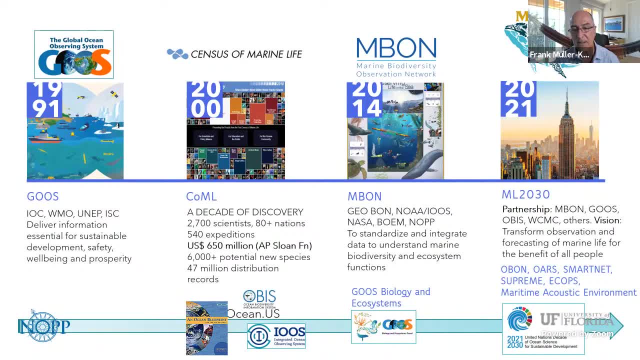 It's kind of more of a presence absence effort, just because we didn't have enough information even about what was living where, And that ended in 2010.. A lot of people were sort of left out. you know, the program ended and nobody wanted to support it or to support a follow on. 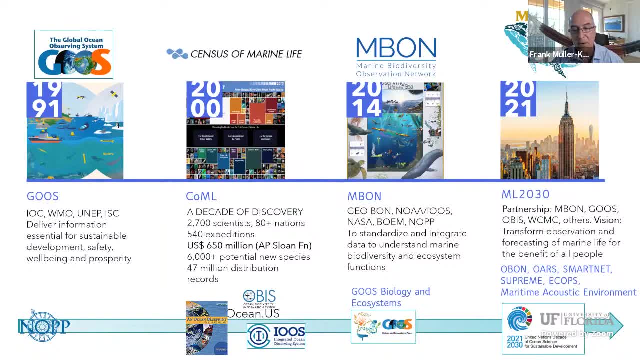 And yet other agencies, especially NOAA, NASA, NSF participated as well. BOEM Navy decided in the US that well, we need to stand something up, And so they had a series of workshops and stood up something called the Marine Biodiversity Observation Network. 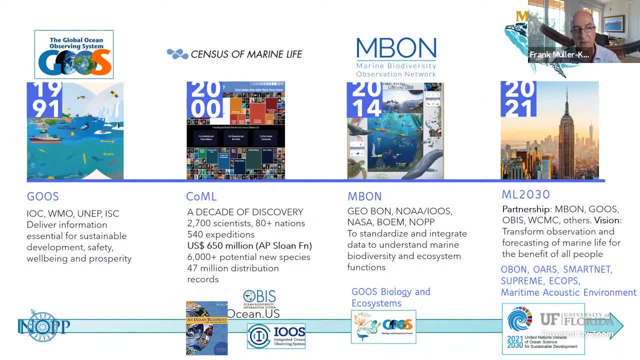 That was happening at the same time that GOOS, the Global Ocean Observing System, decided to form a biology and ecosystems panel that is called GOOS BioEco. same time, 2014.. And internationally, the group on Earth Observations called GEO- that's a kind of a parallel structure to the United Nations- decided to also stand up a biodiversity observation network. 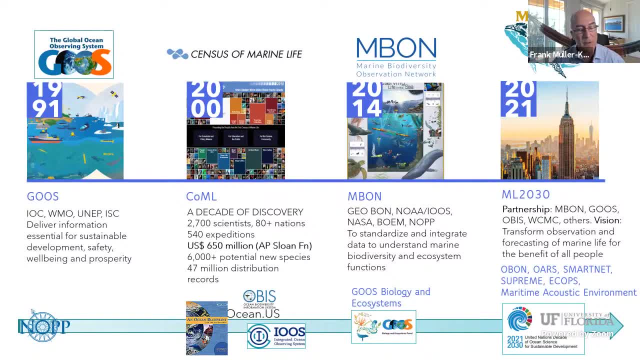 So under GEO bond, we proposed to have an M bond that was already being formalized in the US through funding, And so that's where we are today: We have an M bond that is active. It's funded. There's a call for proposals out in the street right now, with proposals due in December in the US. 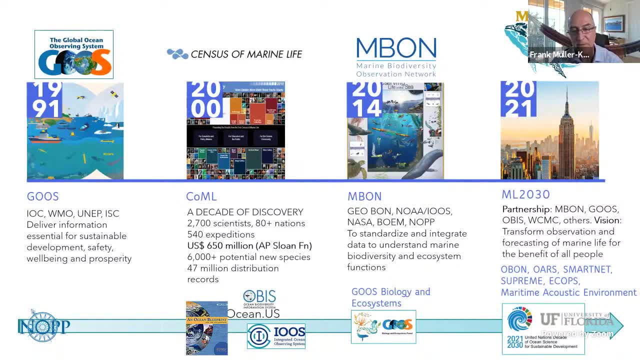 And there's an international framework. So a lot of the effort is to try to convince people that we need to use standards for measuring biological Properties of the world and using standards for data formatting and sharing the data, which has historically been a problem for biologists. 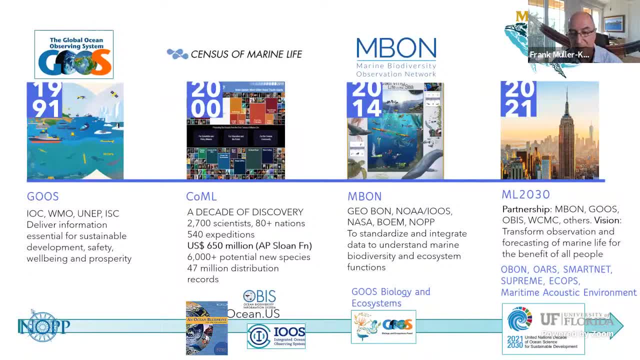 So now, in 2021, we noticed that a lot of people saw M bond as its own thing, you know, and we said: wait, we don't want to be under M bond, which was never the idea. M bond is a networking mechanism and not an umbrella. 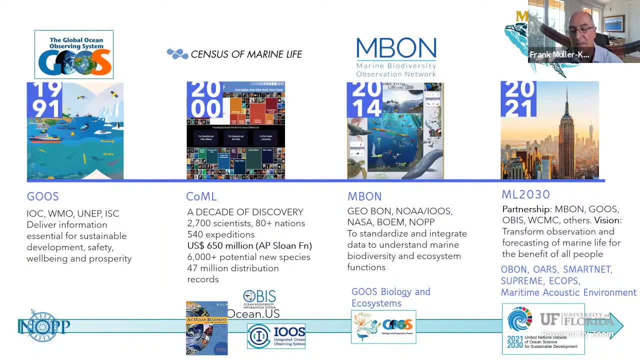 So we decided to work with the ocean decade and propose marine life 2030.. So marine life 2030 is another effort to try to bring people together. There's a lot of partners, including the ocean biodiversity information system and UNEP, the world conservation and monitoring. 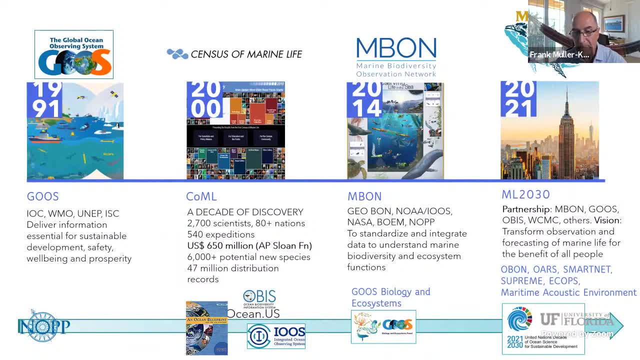 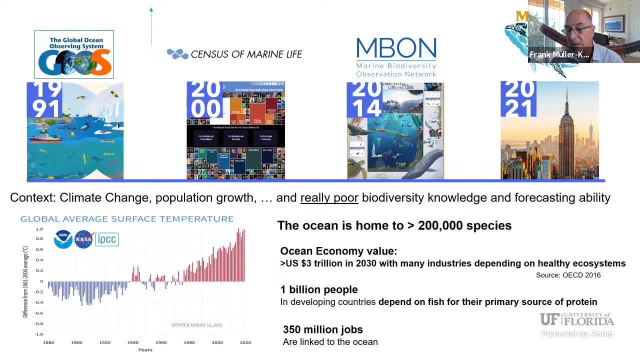 Center and many others. And we know why we need to do this: because the world is changing. We know the world is warming up. We don't even know how many species there are. We know that there's. we have looked at, counted and described about 200,000 species, but we think that there's over a million species in the ocean, mainly bacteria and microorganisms. 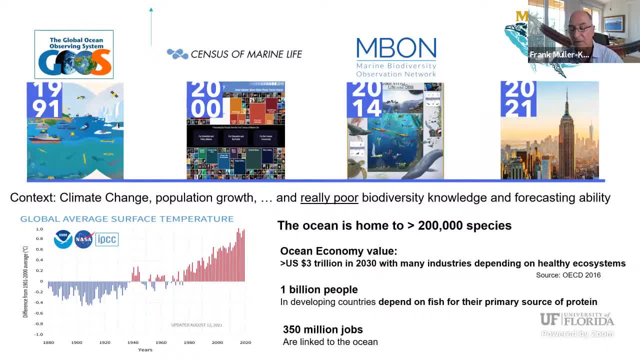 And and yet we don't, we don't know that, we haven't, we have not been able to describe it. So The, the the ocean economy is important. We, a lot of people, depend on the ocean for food and jobs. 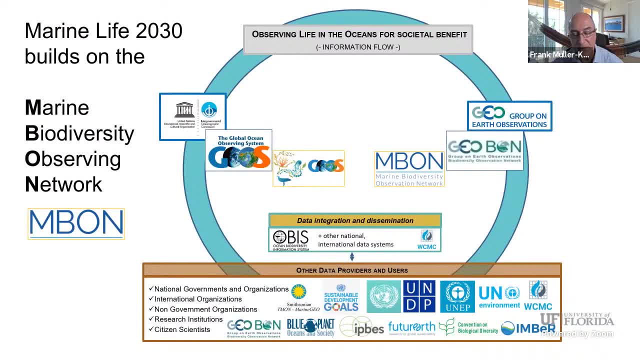 So what M bond and marine life 2030 are trying to do is organize these different international groups into something that makes sense and have people talk to each other about organizing the observations of life in the sea. So I described one process on the left-hand side here that is, under UNESCO, that which is really broader. 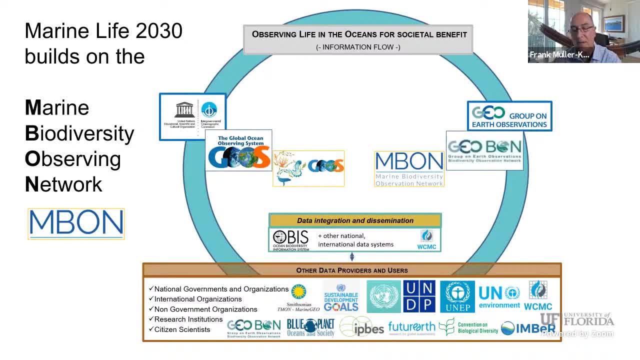 Because it brings in a lot of other UN groups and we have this group on the right-hand side, which is disconnected from the UNESCO and UN side, but it's also it. it involves over a hundred countries and it's called the GEO. 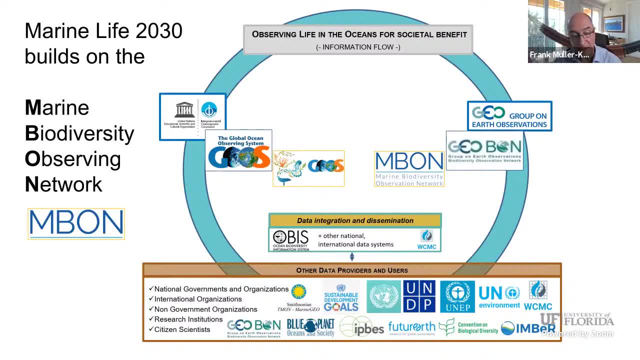 So we're we have a lot, of, a lot of my time is spent in meetings trying to get these two groups together, And I don't know if, if, if you want to get involved, but I welcome you, Because this is a mammoth job and it needs a lot of people talking to each other to generate the data that we need in order to be able to forecast living resources. 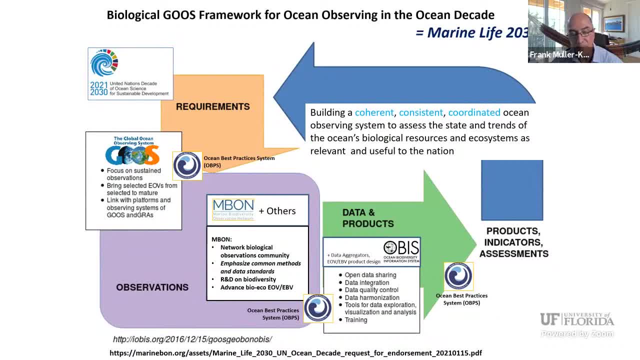 The way that we do that is, we have this framework for ocean observing. that is part of what goose developed already 10 years ago And it's it's kind of on the left-hand side. So goose the global ocean observing system works to to set requirements. 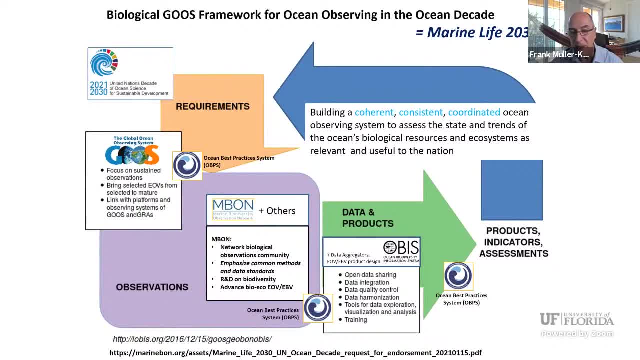 What do nations Need, What do international agreements need, What do individual groups that in any County or city need about the ocean, be it physical variables or chemical variables or biological variables? So these, these, uh, these variables, which they decided to call essential ocean variables are, are kind of coded in a series of spreadsheets where the you, you, define the specifications. 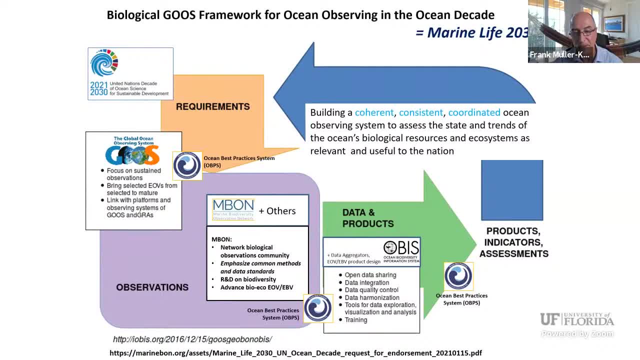 Of what it is that needs to be measured And the kinds of things that need to be measured. in Enbon, What we do is we try to network the community to around certain standards- uh of how you measure things and then how you walk data into, uh, into open data platforms like OBIS. 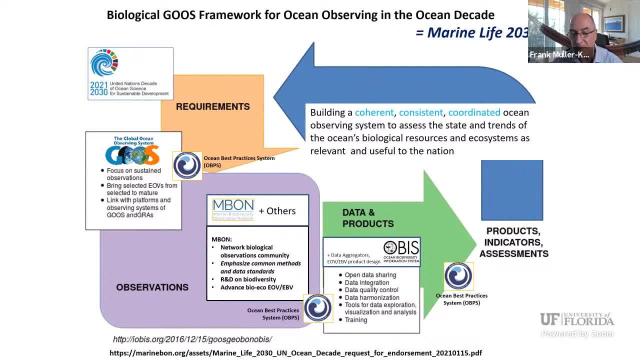 And so the the ocean biodiversity information system. there's another another one that we use, called GBIF, the global biodiversity information facility. These are open databases where people Are that are willing to share the data, deposit them in various structured formats. 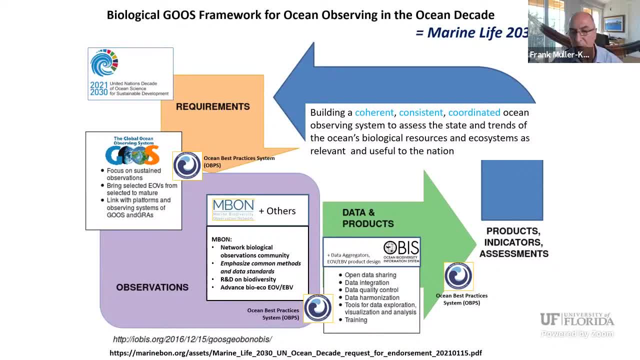 And these formats are quite comprehensive. They go way beyond just documenting whether a species exists or doesn't exist in a location. You can quantify time, place, uh, abundance, productivity and also some of the environmental variables, or have a link to another database in the OBIS records. 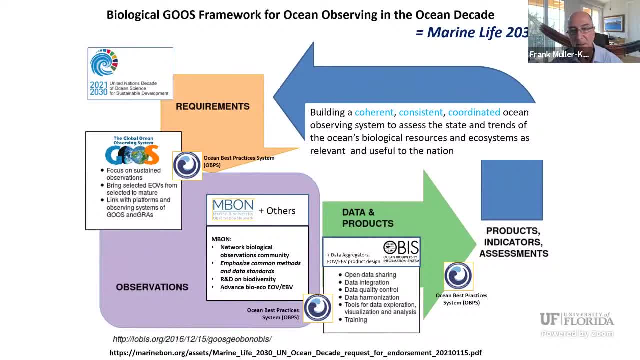 These OBIS records are called. they're formatted using something called Darwin core, the Darwin core standard, And so it's, it's useful if you, if you're a biologist, that you understand that the one way that we can make machines talk to each other. everybody talks about artificial intelligence and how machine learning. 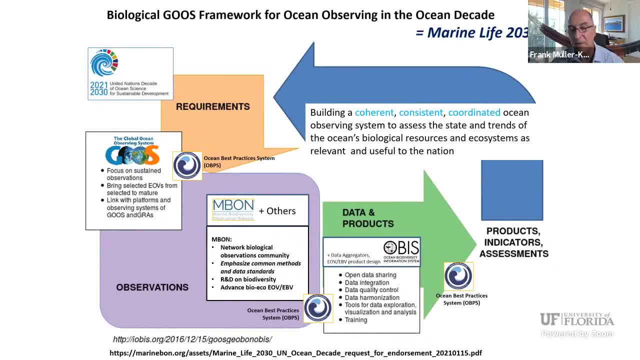 But if the machines cannot learn about a data set, then we're toast. So one thing that we need are standards on how you walk the data around, And that's what, uh, we're trying to work with with these different groups. 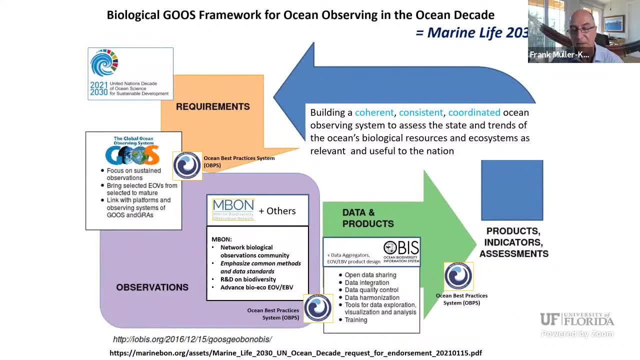 So there's the ultimate intent is to generate products like indicators or indices That people can use about the status of a resource and track it over time. Ideally have these indicators in the form of maps, where you can have stacked maps of physical, chemical and biological or biodiversity properties. 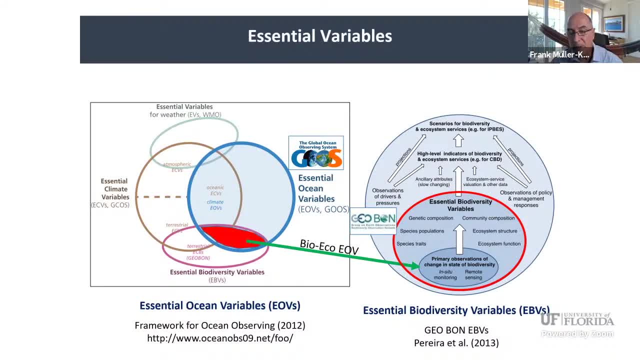 The idea of essential variables came from the climate community, The, the. you may have heard about Essential climate variables, And so this was probably about 10 years ago, 15 years ago, uh, and everybody thought that was a good idea. 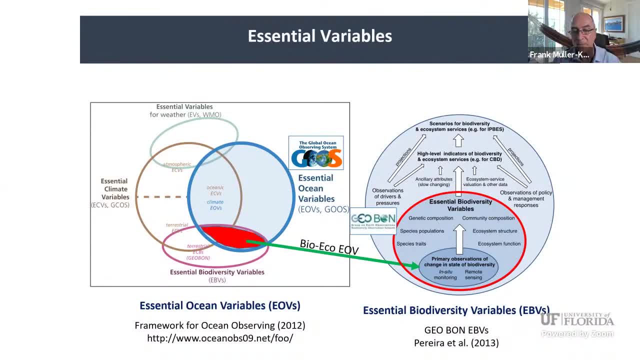 And now all of these variables are trying to people are trying to get them together because they really hang with each other. So essential climate variables are things like air temperature, ocean temperature, precipitation, things that you use to track the status of climate or the state of climate. 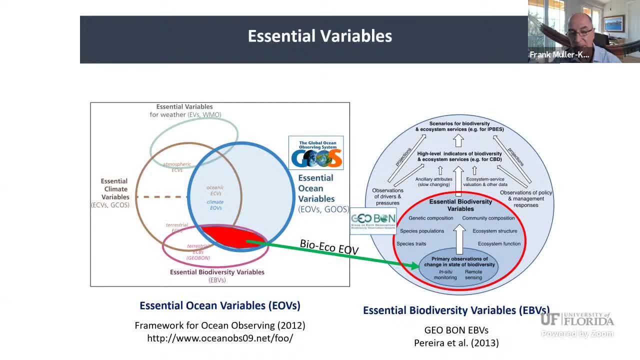 The global ocean Observing system deals with the essential ocean variables, or EOVs, And there are these different panels that, uh, there's a physical panel, a chemical panel, a biological panel, and they, they work with each other, because nobody pretends that you're going to just measure zooplankton and that's it. 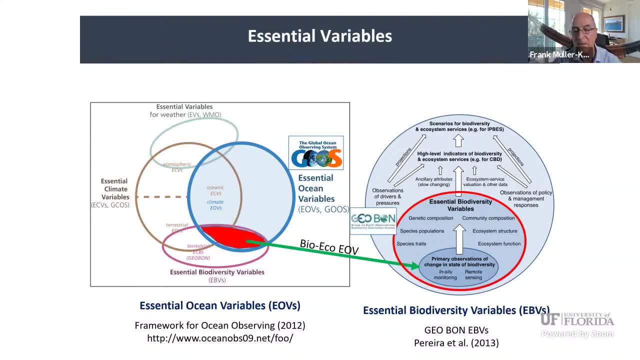 You have to measure some physical quantity or biogeochemical if we want to understand the world. Now, another group that decided to establish Essential variables is this geo bond, The group on earth observations, And they came up with the idea of essential biodiversity variables. 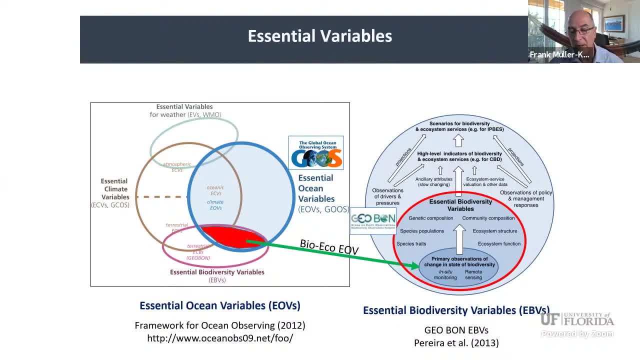 And so there's a. there's a lot of buzz. There's also a lot of confusion around about what these things mean, And the essential biodiversity variables is nothing but maps or stacked maps, basically data cubes of essential ocean variables for us in the in the ocean community. 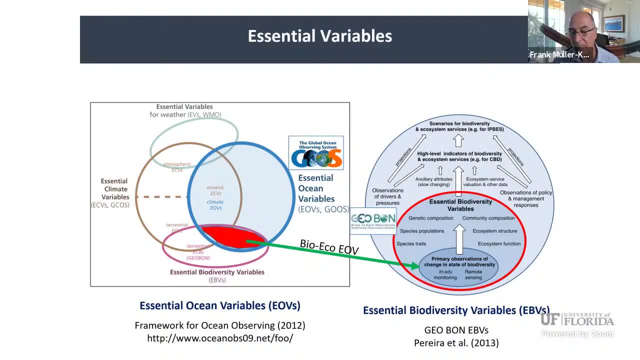 So, if you think about it, uh, if you can make maps, Yeah, Of genetic composition or species distribution or species traits, and have time series of them, then you have an essential ocean, essential biodiversity variable, or EBV, And that's what we need to derive these indicators. 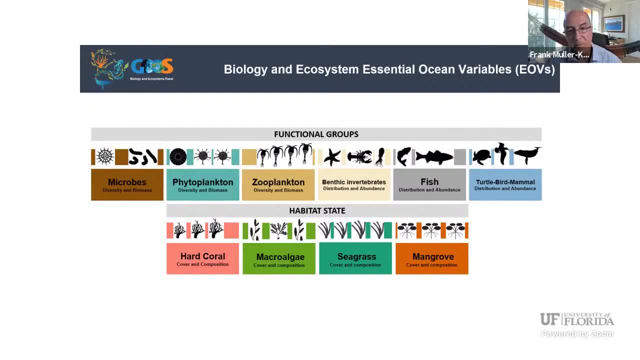 This is what we talk about when we um, when we talk about essential ocean variables for biology and ecosystems, and it's these, these. I'm not telling you that these things are different. I mean they. We're just trying to organize the community to talk the same language around standards and stat, especially if we're going to measure these things. 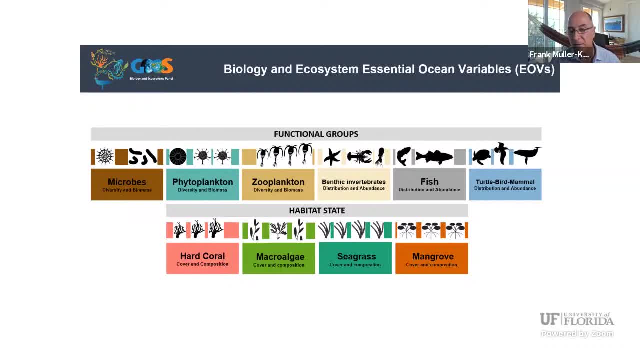 In an operational way. So if somebody in a country X decides to stand up on an observing system, they can go to a cookbook scenario and say: for this problem, you can measure these different essential ocean variables and you may have an indicator about the conditions of your, of your resources. 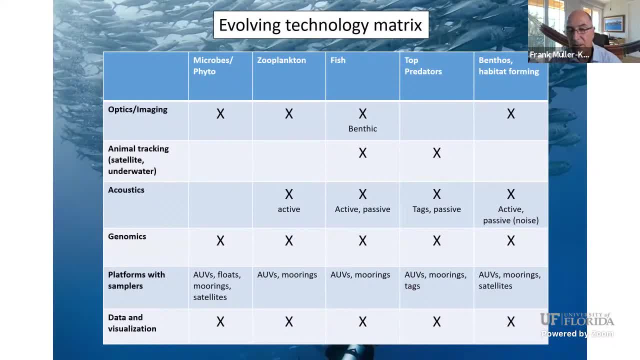 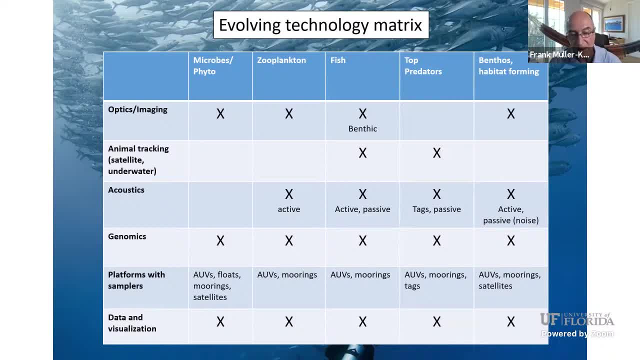 uh, uh, uh, uh, uh uh. or eDNA, which allows us to do a lot of things very, very quickly, but it's still quite expensive, And doing this with automated samplers. Ultimately, all of this has to come together in databases, and so we're pushing for visualization and uh and and data science concepts. 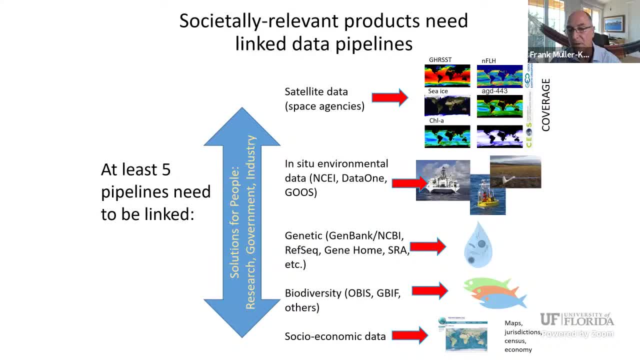 So all of these databases have to be linked together. We we know that there's an enormous and easy access to satellite data, But even all the satellite data are different. The temperature satellite data is different from the sea ice data, from the wind data and precipitation data. 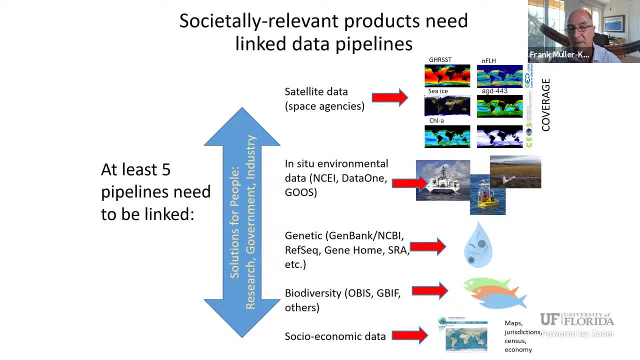 And so it's a mess for people that are trying to use these. If you don't know anything about managing large quantities of data, or if you're a resource manager that wants to use some of the these uh data sets to understand what's happening, 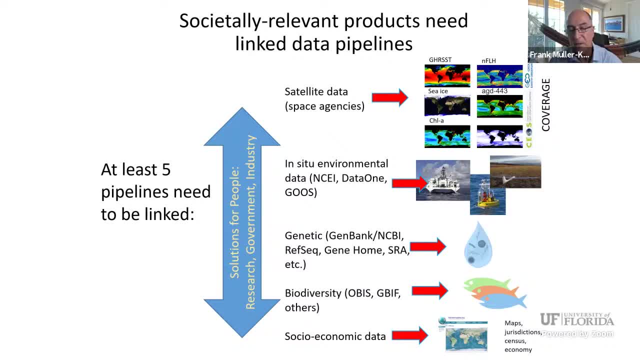 A lot of other data, field data, goes into what we call these databases, And there's some, like the NCEI, that is managed by know our data one, uh. but there's a lot of different databases out there and most of them are not connected to each other. 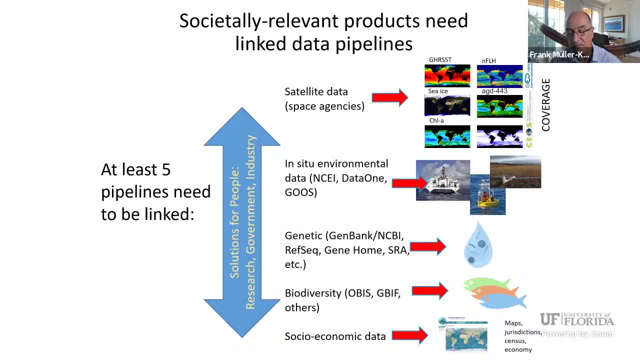 So it's a mess. You have genetic data going to to the nucleotide databases like GenBank here in the US, but there's others around the world And while those are linked with each other- the nucleotide databases- they're not linked to to biological databases like OBIS or GBIF. 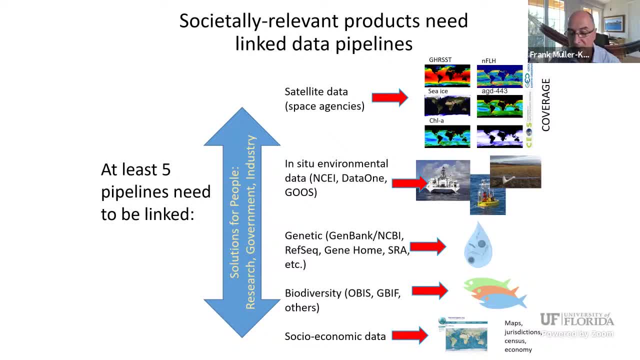 Or the NCEI. So that's one thing that we're trying to do. Ultimately, you want to link this to socioeconomic data, which is always the last frontier, And it should be the first thing to consider when we're doing this. 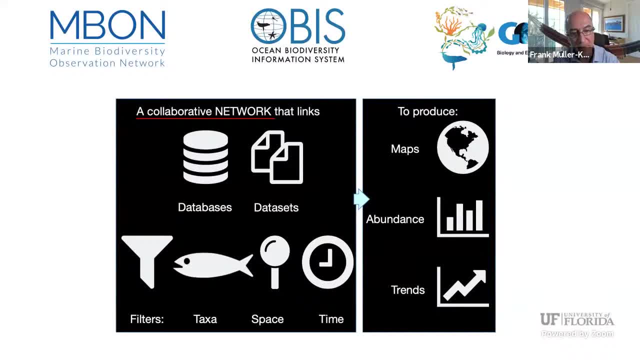 So what we're trying to do is the, the, the, the framework for establishing databases that host data sets in standardized fashion that include taxa, with tax for space and time, So you can make maps. So you can make maps. So you can make maps, track abundance and and, and look at trends over time. 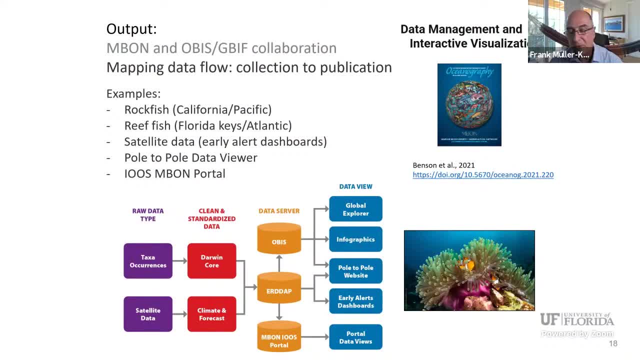 We have, uh, all of this seems so, um, intuitive, but it isn't. We're trying to organize this through this diagram in the bottom, which was just published just a few weeks ago, where we have the occurrence of organisms stored and databases using the Darwin core format, which is kind of a parallel to the. 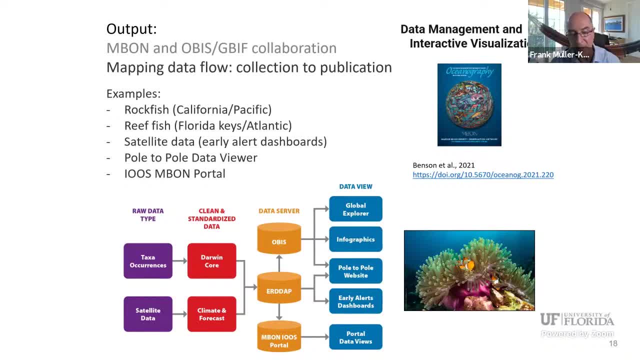 Cdf Or net CDF data structure for climate data, even though you can store Darwin core structures in net CDF file formats and we store them in data servers and serve them through the same sir Services, Like bird up, that you use to serve climate data or weather data and then use the viewers that we have on the right-hand side of the diagram. 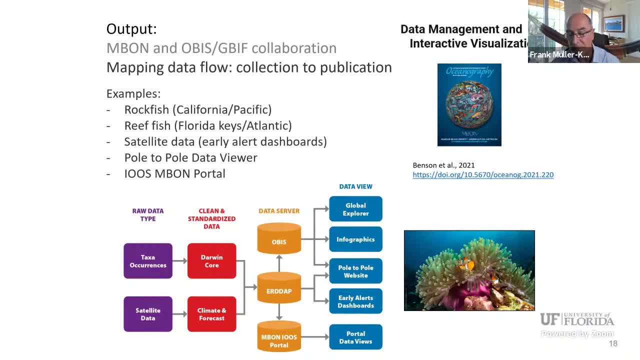 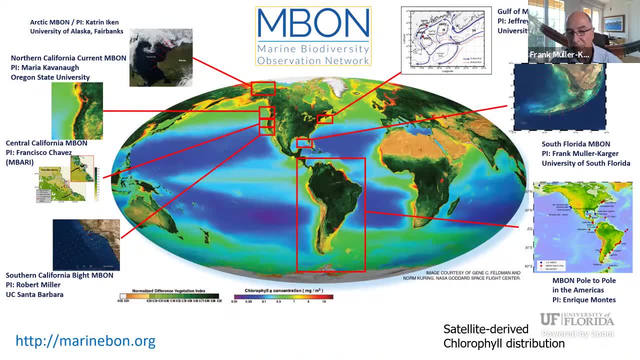 In many cases we're trying to cook up very, very simple infographics and I'll show you an example of that later on. So the MBON projects right now around the US cover not everywhere, but we have some healthy coverage on the west coast of the US. 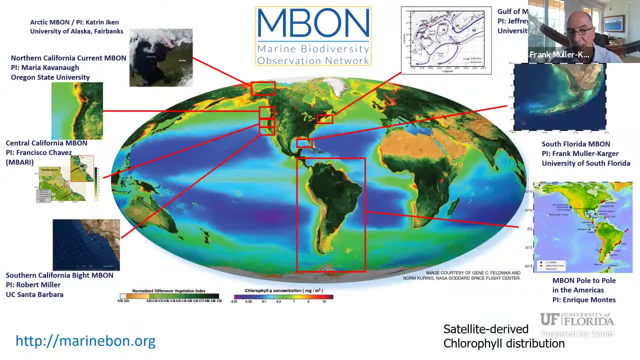 from California to Oregon, all the way to Alaska. The Alaska group is looking at the Chukchi Sea And on the east coast we have a group looking at the Gulf of Maine and we have our group looking at the Florida Keys. 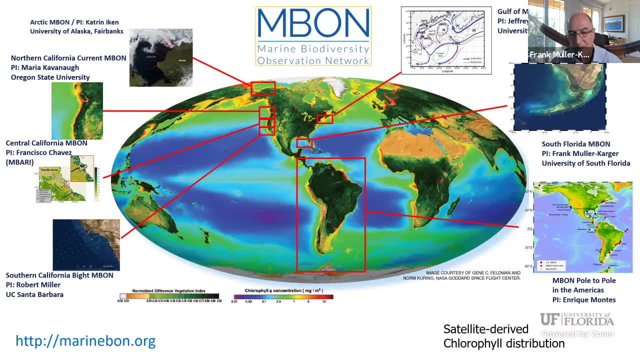 We also have a group looking at what we call the pole-to-pole MBON, which is trying to work with especially groups in Latin America and working on standard observing methods for sandy beaches, rocky shores and satellite data. all of that to put data into the open data sources. 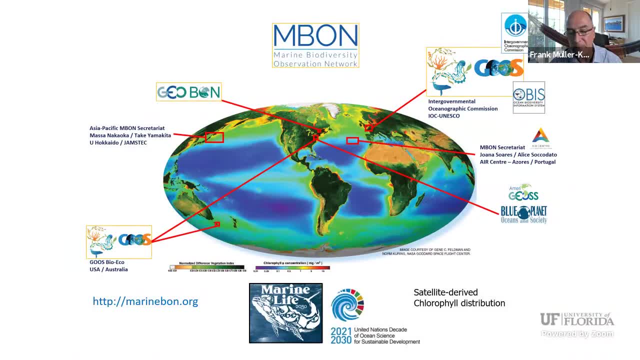 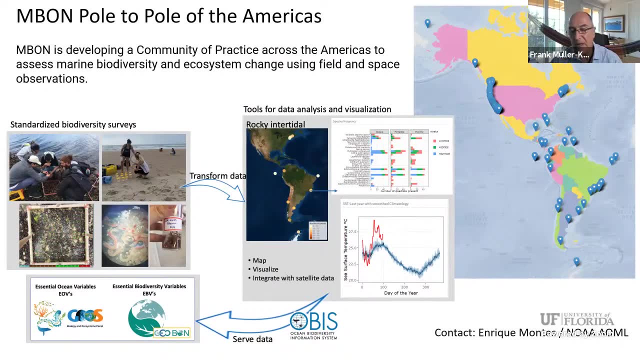 And we do that working with the groups that I've mentioned, so I'm not going to spend time on this. So some examples. the MBON pole-to-pole to the Americas, has a graphical interface. If you look it up, you'll find this type of device where people in different places can easily 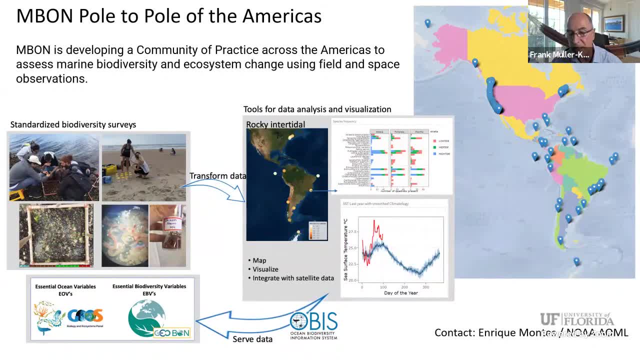 they can click on their station and they can get a download of the satellite data, the historical data from OBIS, and they can input their data as well to see how it looks in context of other data set. In Florida we have a very interesting, very interesting project. 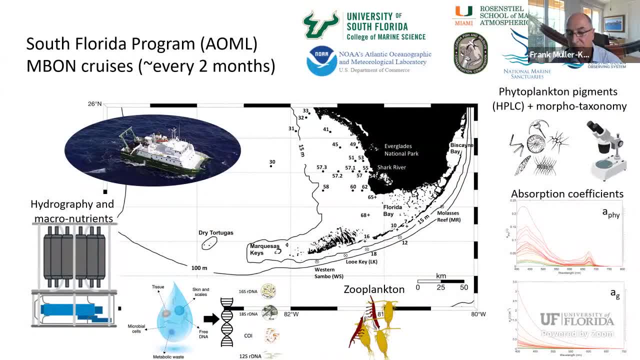 which is called the M-BON South Florida Program. We go out on a ship every two months. We do this jointly with NOAA, AOML and the state of Florida with the Fish and Wildlife Research Institute. There are several other groups involved. 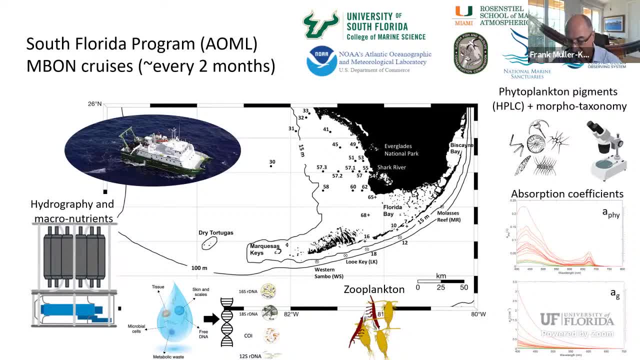 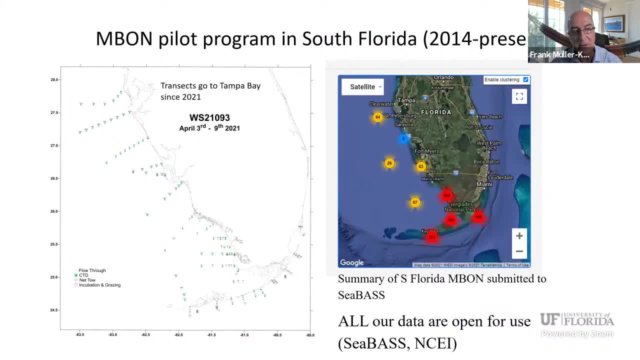 Our cruises go out of Miami, go along the Keys and then they come up the west coast of Florida. Basically, this past year we started going up to Tampa Bay because there were red tides that were recurrent and we wanted to make sure that we covered those as well. 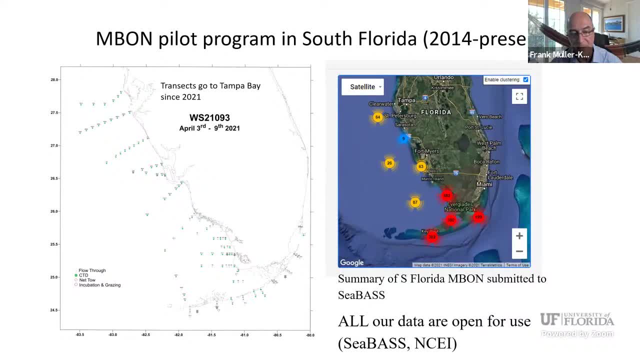 So we're working with the state of Florida and the red tide group there as well, So this data is all available. We put our data as quickly as we can, at least our data, and not everybody on the cruises shares their data, unfortunately, but our group shares all of the data. 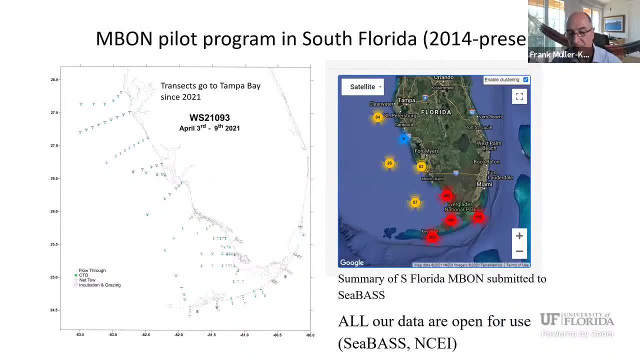 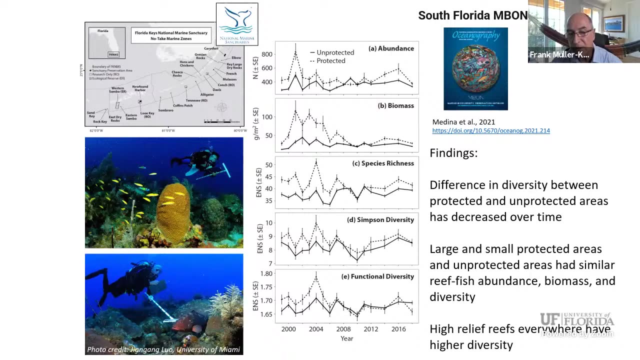 Everything from pigments to the DIC data, to nutrient data, to the optics data that we collect and we put it in open databases as quickly as we can. An example that we did with the M-BON project in Florida is try to look. 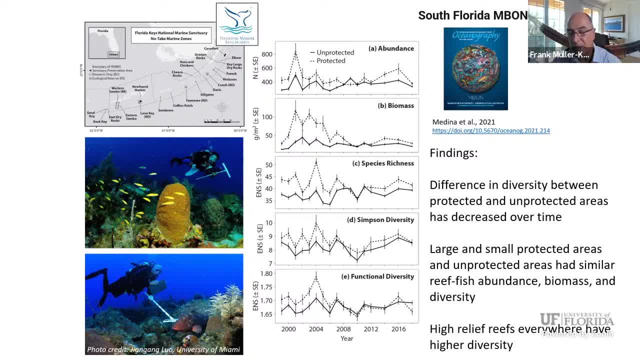 at the reef fish variability in terms of species abundance and so on, And these are some of the results we just published- is that we find that, unfortunately, over time, the protection that no take areas afforded to fish in the Florida Keys has sort of decreased, or the amount of fish. 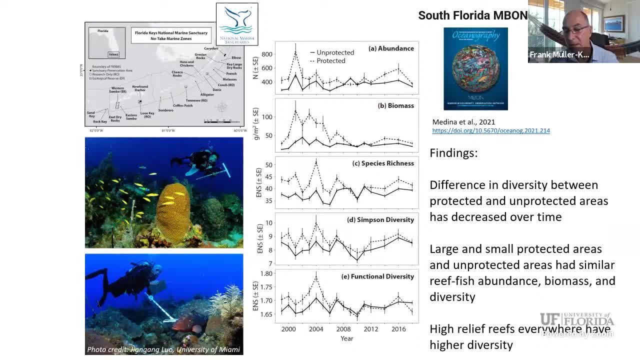 in non-protected areas is very similar now to what it is in protected areas, And so why exactly this is is not completely clear. But it turns out also that larger protected areas in the Florida Keys are just as effective as small ones, And we think that the problem is that one is that even what we call large protected areas 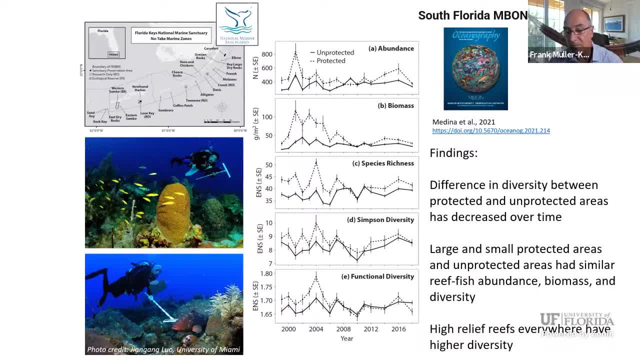 like the Florida Keys, which is a very large protected area like the Eastern Sambo Reserve, is still too small because the reserves are not big enough to protect the diversity of these fish And, as most of you know, even though coral reef diversity and cover has stabilized, 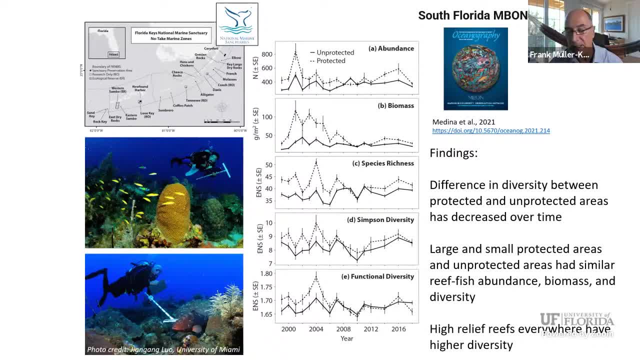 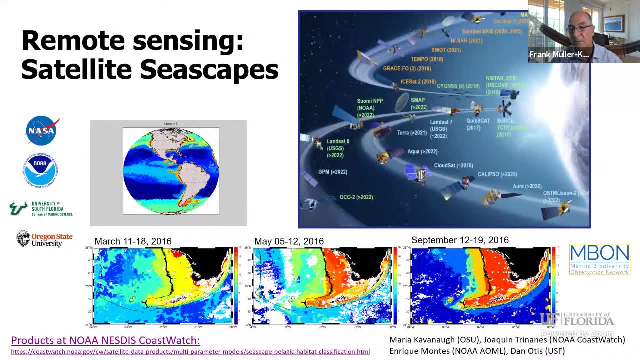 over the past few years there was a. it's nothing compared to what it was in the 1970s, So there is a big issue on looking at biodiversity and the resources in these areas. We're also using satellites, but whatever satellite you can think of, we are using it. 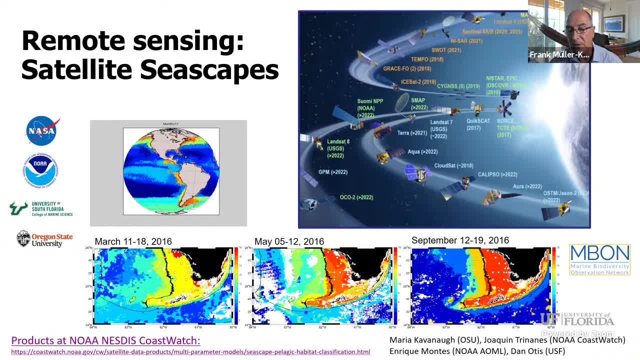 to look at biodiversity and the resources in these areas. We're also using satellites to look at how do we classify biogeography in the sea, and not just as a static map like we used to have in atlases before. but how does this change historically? 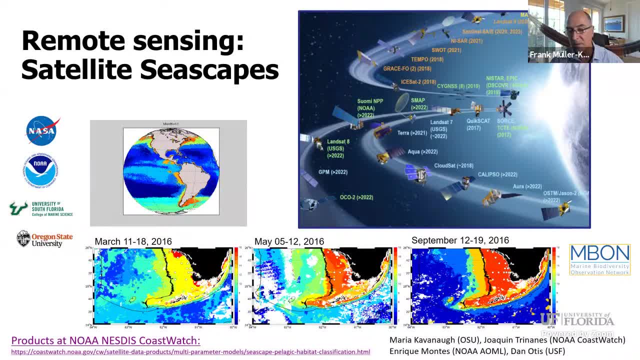 Can we track trends in biogeography in the seas And we developed this that we call seascapes with Maria Cavanaugh at Oregon State University. So those are now operational. They're served operationally through NOAA Coast Guard And those are now operational through NOAA Coast Guard. 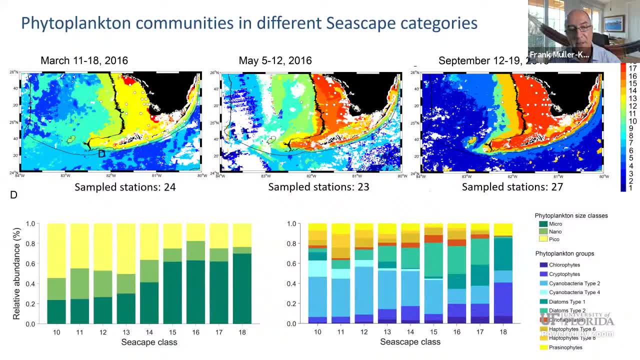 An example of that is using our is. we're comparing these seascapes with what we collect on board the ship, So we're trying to see if these seascapes makes sense, And so one of the ways is comparing it to phytoplankton groups. 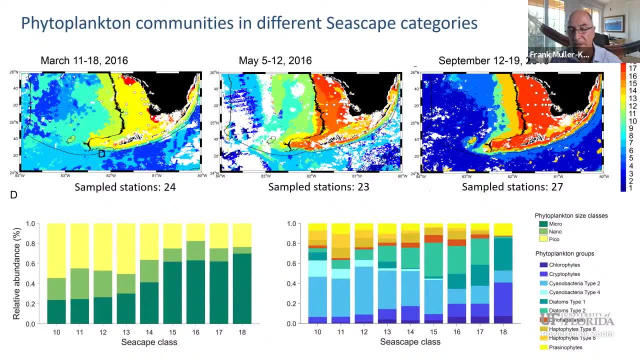 And so we find that there is some correlation: smaller phytoplankton being farther offshore and bigger phytoplankton living near shore And people California and doing that with fish. Some other groups are trying to do that with marine mammals. So there's a big effort with many people trying to compare acoustics, fish concentrations or 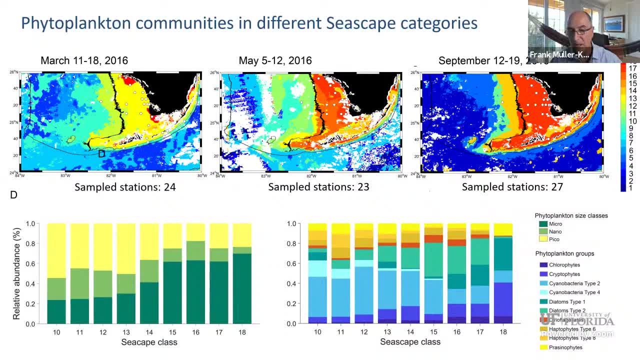 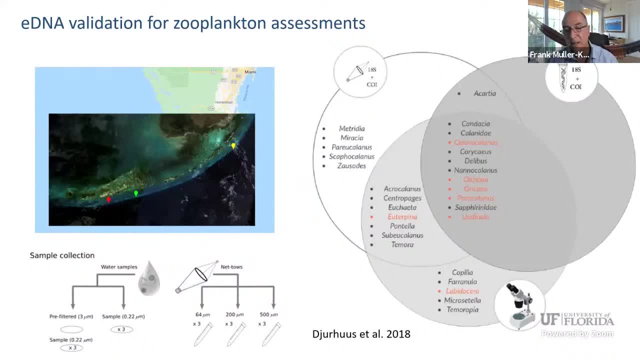 abundance in phytoplankton or other types of plankton and how that tracks over time with seascapes. We're trying to do that with eDNA also and even comparing eDNA assessments with acoustics in the Florida Keys. Now we have a time series of eDNA measurements in the Florida Keys. 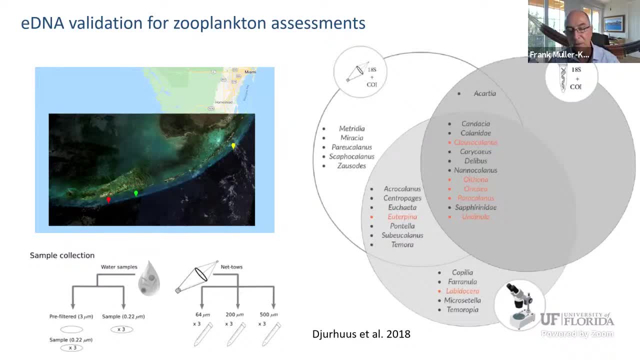 This is an example that Annie Juras did, where she compared the traditional ways of counting zooplankton using, for example, microscopy and from eDNA, And we find that it's not always the same, but the eDNA gives you a lot more information than you would normally collect with other methods. 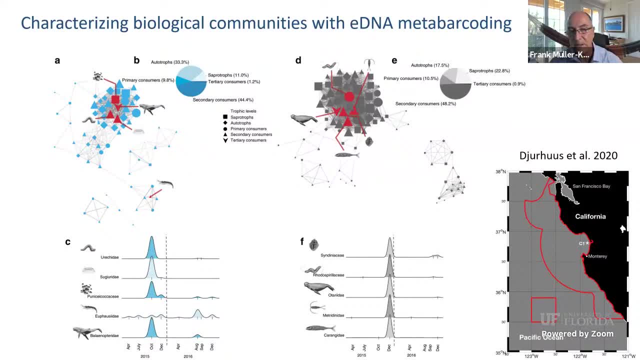 You can even find ways of. we did this comparison between the Monterey Bay and Florida and the Florida Keys. There are two sanctuaries we work closely with National Marine Sanctuaries where you can look at associations between groups of species using eDNA data, And we try to put all of this. 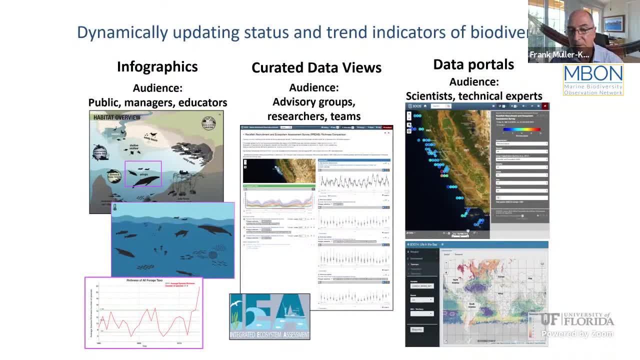 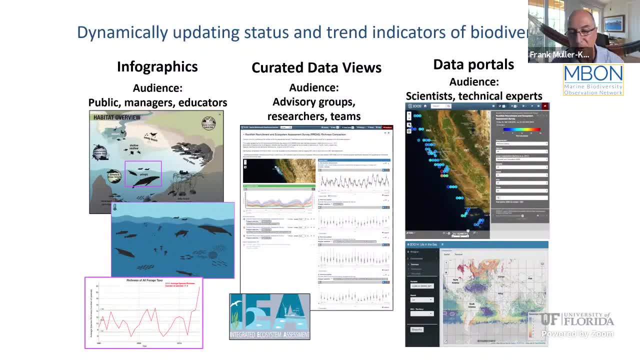 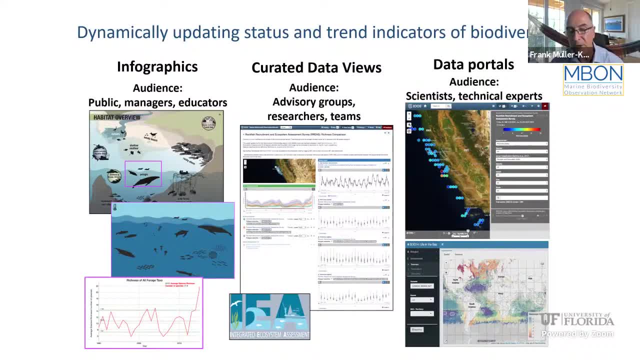 they don't have time. They're trying to work sanctuary permitting and other programs that they have, And they just don't have time to do a data analysis that is as deep as a scientist could or as a student or a PhD or a postdoc could. So we need to present the data to the public in a way. 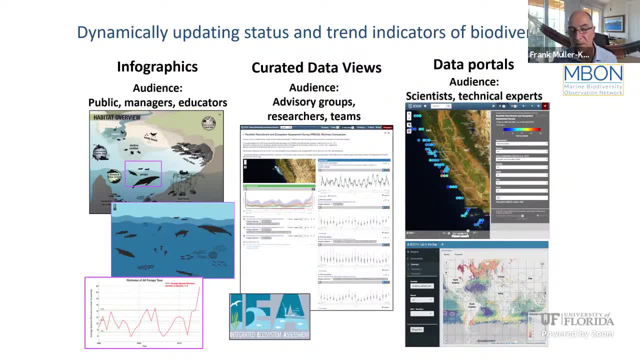 that is much more accessible, And one way that we found to do that is through these infographics where we have cartoons of the environment And, for example, you can have a coral reef or a seagrass or a kelp forest annotation and some organism that 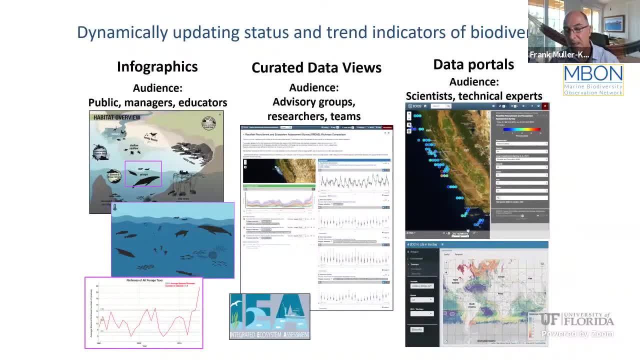 they may be interested in And if they click on it online, that links to the data And it's a data set that gets updated regularly And so they can look at it year after year or every time that a data set is updated. they would get that And that's linked to the satellite. 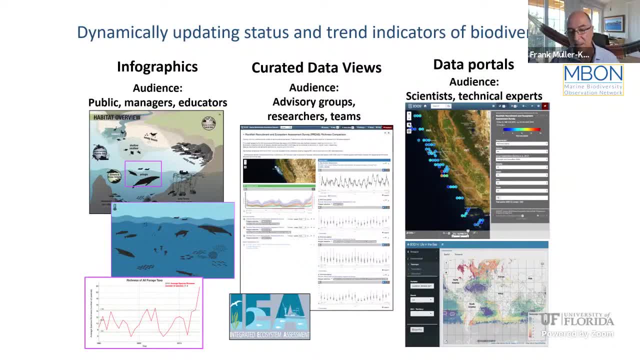 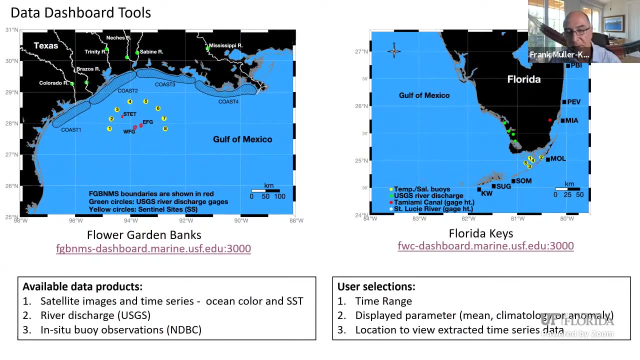 Data record, like temperature, chlorophyll, seascapes, and they can get these a series of time series in a way that is relatively understandable. We're also doing these dashboards in the Gulf of Mexico. We're doing that for the. flower garden banks because there was an event that they detected mortality And the coral reefs, as far as we can detect, an event where a lot of fresh water from the coast moved over to the flower garden banks, which is over 100 miles offshore, But that was enough. 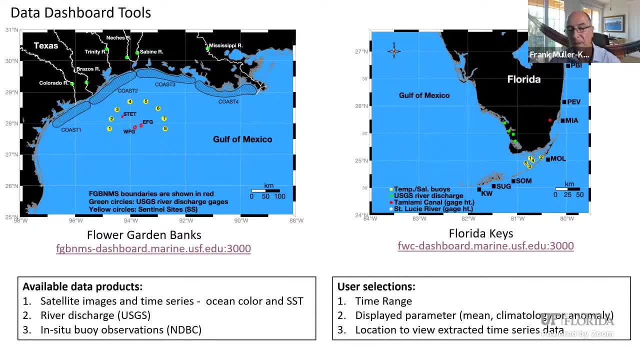 fresh water to cause such a stable environment and a turbidity plume. that caused anoxia on the reef and a lot of corals died, So there It hasn't happened since. but they asked us to do a tool where you can get a kind of an alert based on 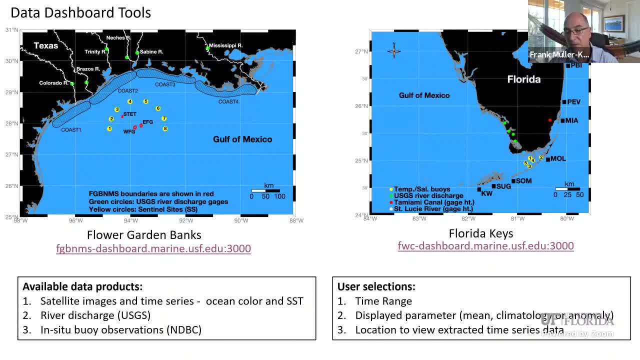 automated satellite data sampling that tells you, hey, you have a turbid water plume coming your way, And so that's online now. And we have something similar for red tides as they wash down toward the Florida Keys, And this is kind of what it looks like. You can. 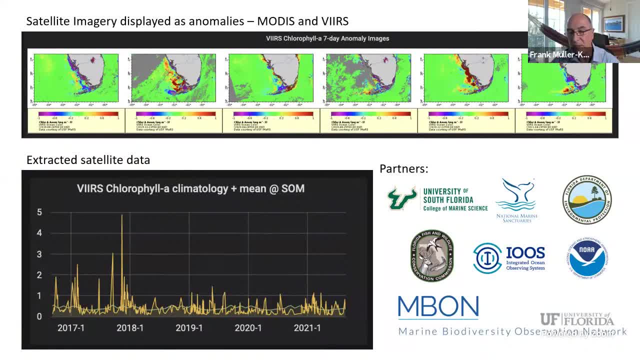 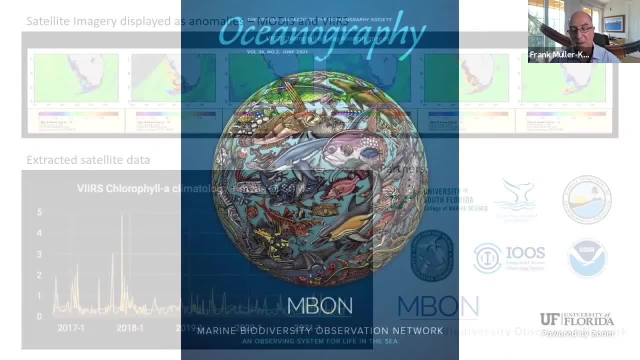 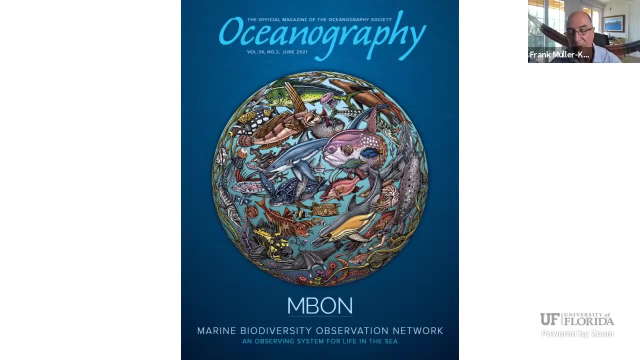 You get the satellite data, you can look at time series and you look at time series of other parameters like the chlorophyll concentration or also river discharge or turbidity that we may have access to. So a lot of these results are coming online now in a special issue of Oceanography on MBON. 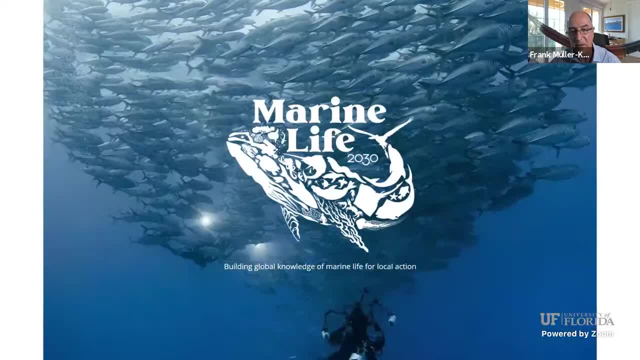 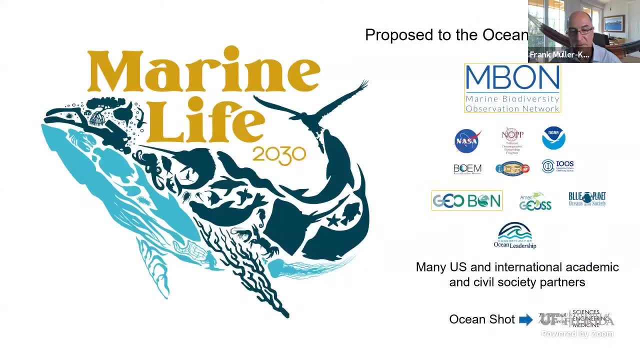 It's just being put together now. Some of the articles are online now and leading up to what we're trying to promote as a marine life effort, And so marine life is the proposal that we have for the Ocean Decade, for which we're inviting now projects. 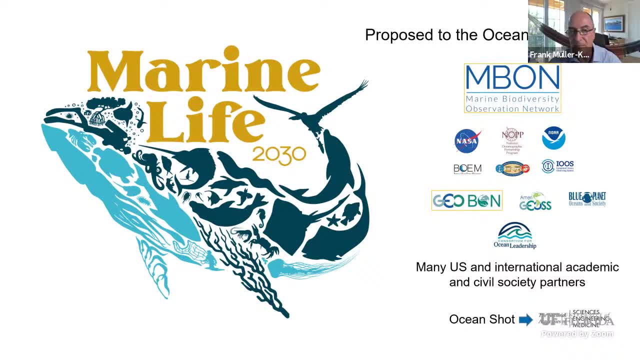 It is, at least in the US. there's a lot of good will, good buzz about the Ocean Decade, But there has not been any funding that the US has put behind the Ocean Decade programs, And so that's something that we're trying to work. 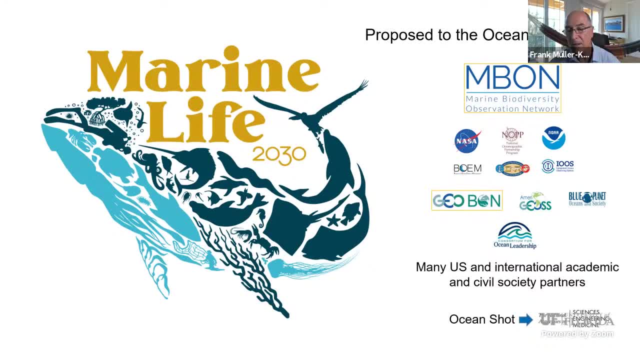 If you're interested in helping with that, it is time to work with your congressional delegation, for example, and say: you know we have the Ocean Decade. the US should participate and you should put money into these programs And, as the budget process that we're going through right now in the US is extremely complicated, 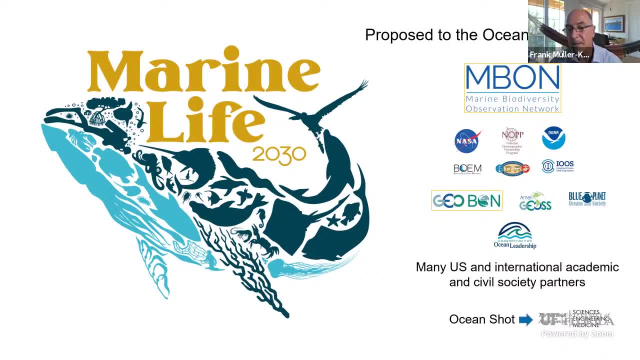 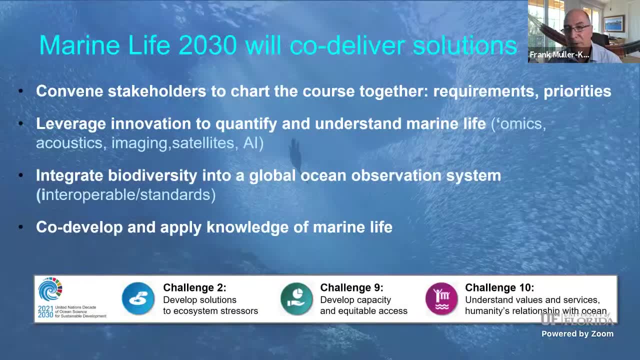 there is still time and there's always an opportunity to talk to your representatives to make sure that these kinds of things happen. So, with marine life, we want to bring people together to talk about requirements, priorities, developing standards, but especially doing this in a way that is useful to people that use data. you know the park managers, marine protected area managers. 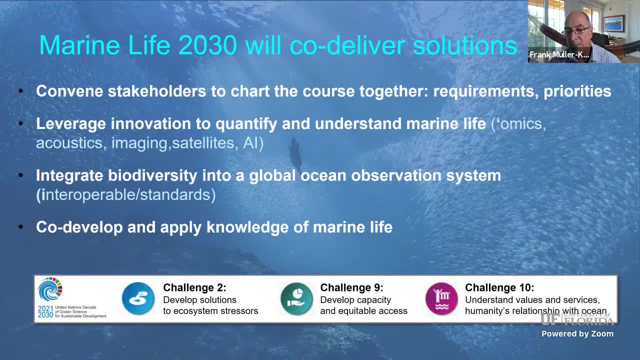 people that are looking at red tides in an operational sense, people in industry that are doing fisheries or aquaculture, or environmental impact statements. We want to integrate biology into marine life. We want to integrate biology into an observing system, a global ocean observing system. 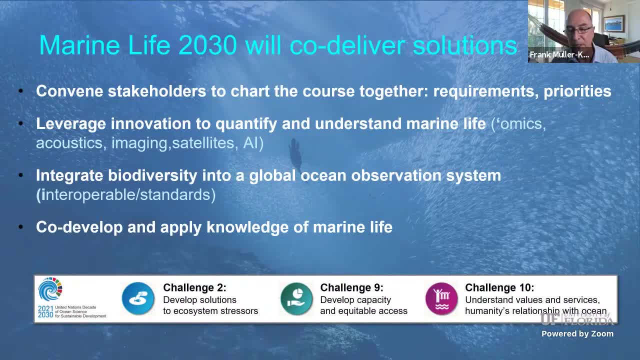 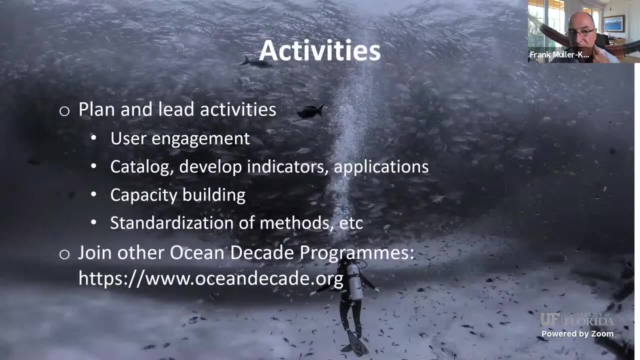 so that we're not only depending on physical data to predict what biology is going to do, without having the biology to verify that or to calibrate the models, which is what we do now. We do biology by proxy, And so we want to establish this idea that we want to co-develop the marine life 2030.. 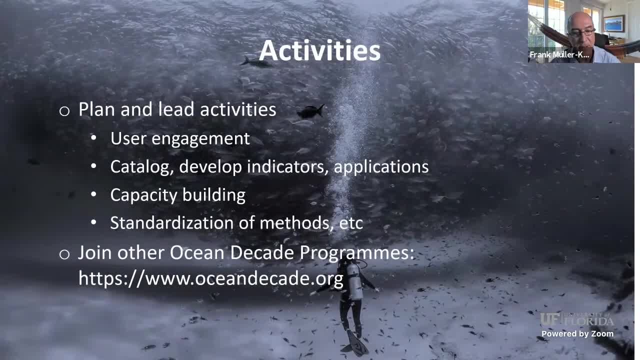 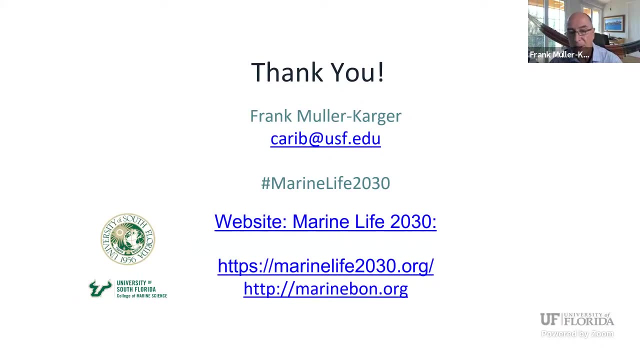 And these are some of the things that we want to do. that we call activities, basically having workshops, Training efforts, continue to work on standardizing methods and getting the community involved in the entire process. So, anyway, if you want to get involved or if you are interested in these kinds of things, please send me a note. 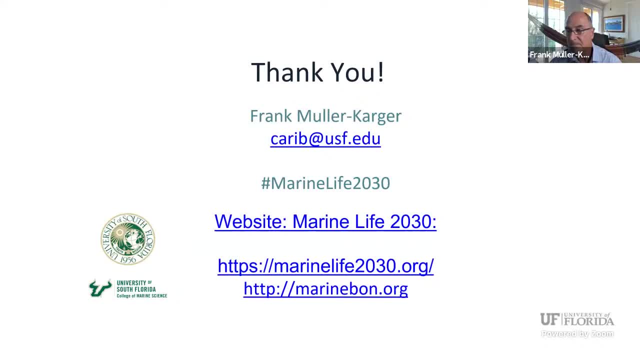 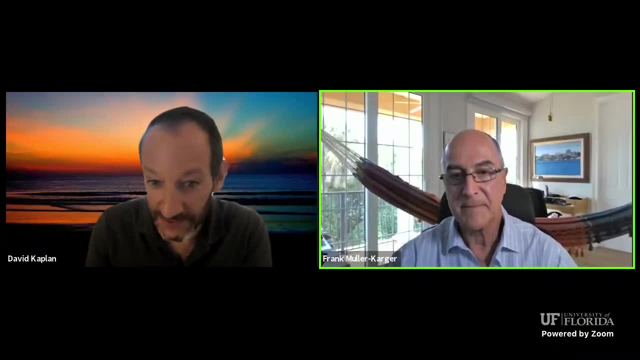 I'm easily accessible at this email. Thank you Great. Thanks so much, Frank. Let's give Dr Miller-Kager a round of real or virtual applause, Your choice here, And we will take questions, Questions from the group here as well, as I'll go check on YouTube. 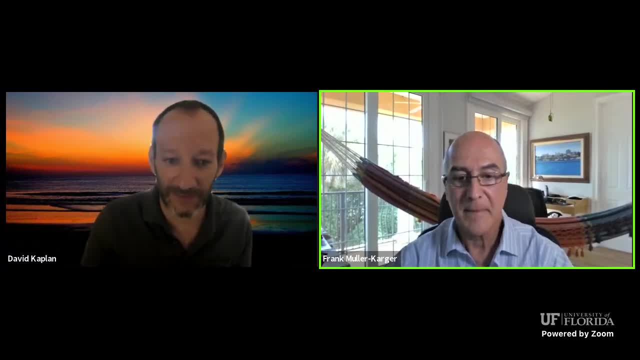 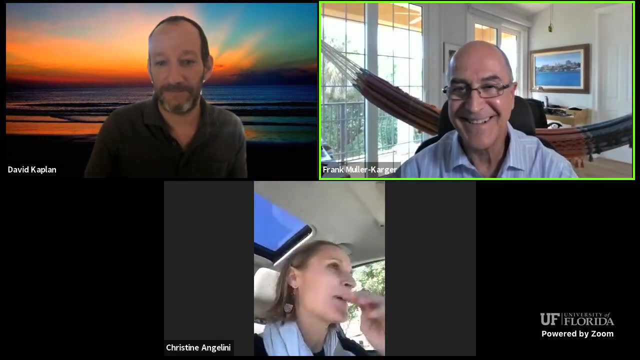 Christine, I see you have a question in the chat, if you're available, Otherwise I can ask on your behalf. Sure, Yeah, Hi Frank. Sorry, I'm going to uncharge a kid pickup today, So I apologize if my internet is a little spotty. 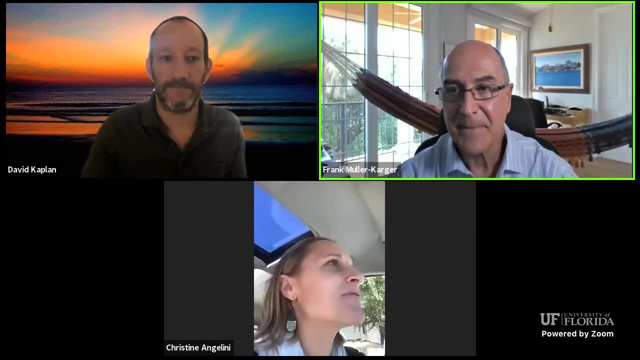 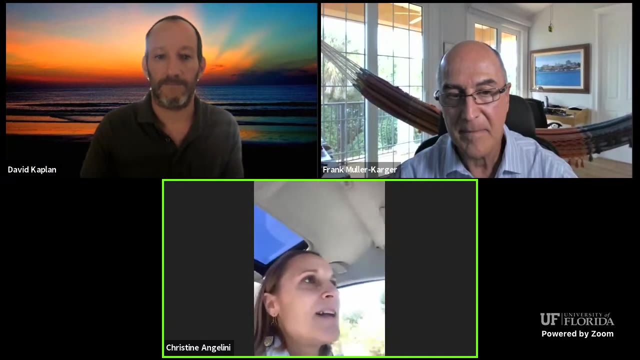 So my question is about the idea of potentially publicly sharing information about some key targeted species, whether that's organisms that could be exploited, like key fisheries and or endangered species, where, if the whereabouts of these organisms becomes more publicly known, it creates an opportunity for exploitation, and whether that's kind of ecotourism and going and looking after whales where we know that they are. 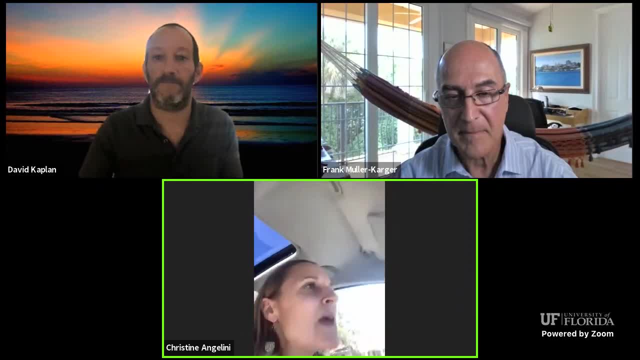 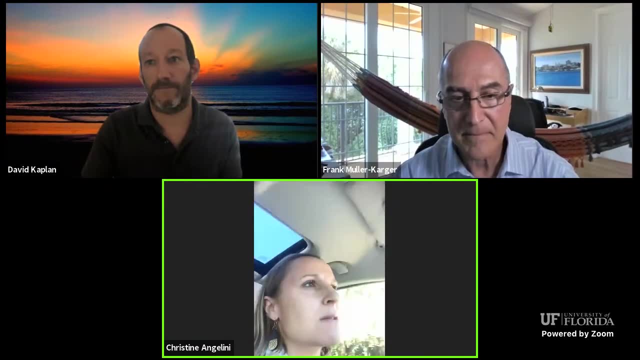 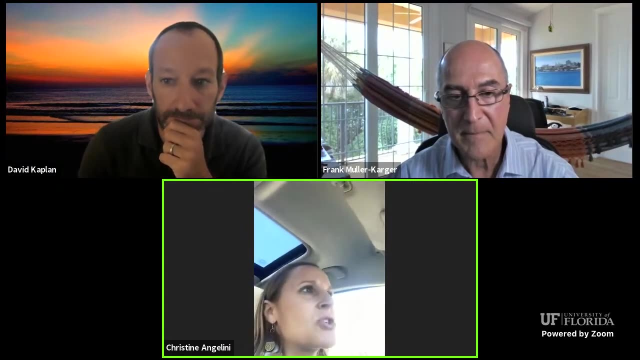 And so I'm just wondering about sort of the sensitivity of of making publicly available some of the data that's coming about from from these biological observations and coordinated networks, and how the community is thinking about if and how and in what ways to share this information with the general public. 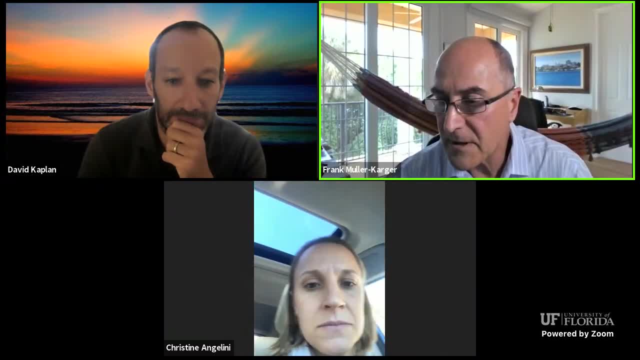 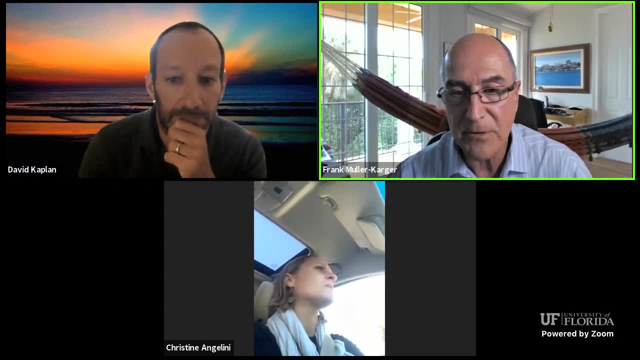 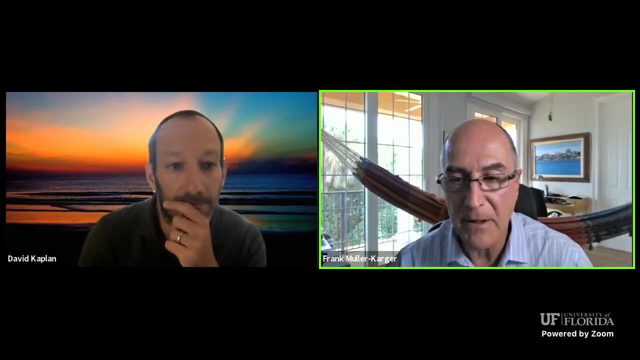 Yeah, well, that's a very, very important question. There are several ways that I think that you can handle that. One is working with industry, of course, and making sure they understand that knowledge doesn't mean just go take out everything you can. 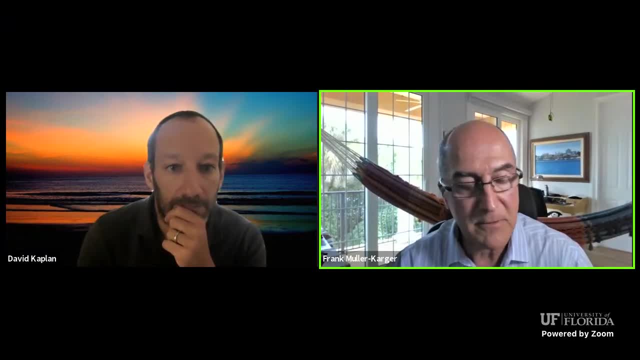 One other way is to synthesize the information. So we're interested in tracking the health of the environment or the ocean, or the health of our population. You don't have to make explicit where you have a specific organism living at one time or where they reproduce like spawning aggregations. 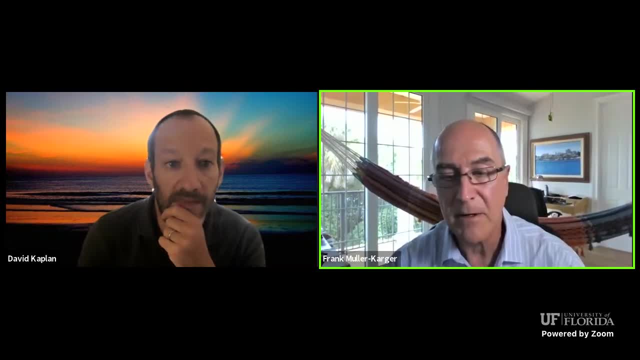 Most fishermen know this anyway, so I don't think that you're gonna be telling fishermen something they don't know in many cases. But what we can help is in track the health of a population. So typically what people do is they share the data. 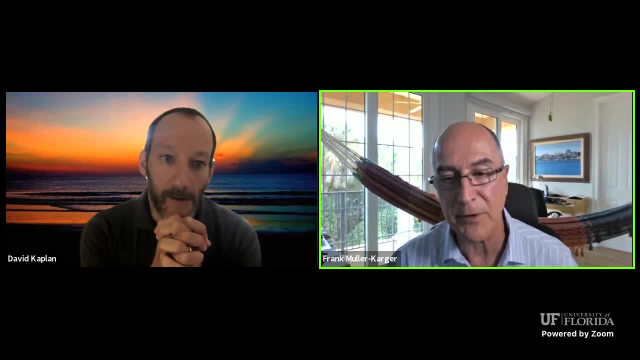 with a data aggregator that doesn't share the original data but produces a product that is constructed with a method that is verifiable if you had access to the original data. So there's. I think that there are ways to do this, Christine, without necessarily encouraging people. 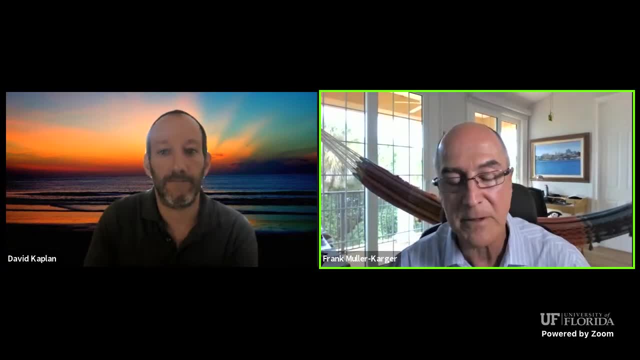 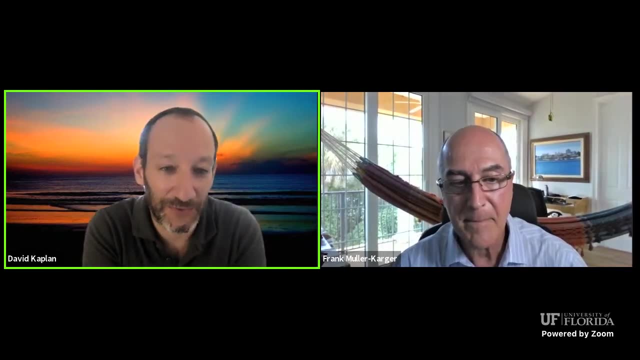 to exploit the resource further. but it is an important question, Thanks, and seeing the global scope of the sort of the goals for the ocean decade, for MBON, it's like at one hand overwhelming, you know, just to think about the great biological diversity that you're trying to catalog and coordinate. 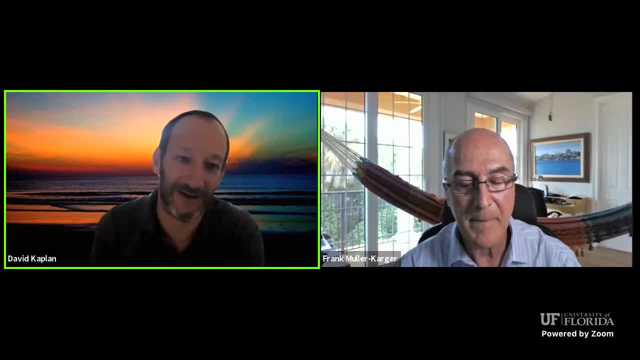 And of course it's a that's also motivating, right, Because if you don't catalog- right- that's a lot of people- and coordinate it now, we may be losing it before we even understand it. I guess my question goes to, like that giant set of data that you and colleagues and all over the hundreds and perhaps 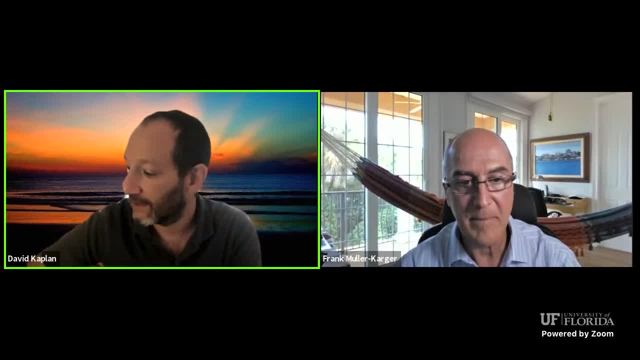 thousands of investigators and agencies are compiling, being so difficult for a natural resources manager to ask questions with. And so there's this intermediary step that you said, of course, with a PhD student or a postdoc or a PI. that's what we love to do, But it also means 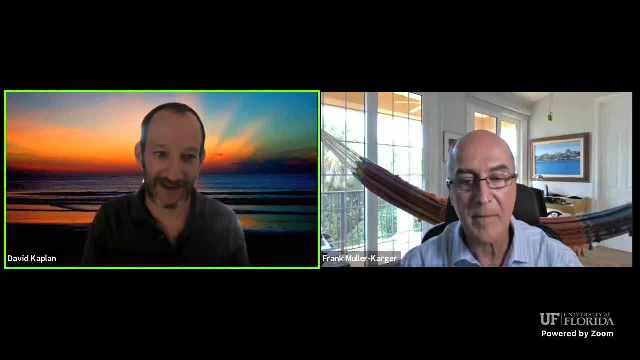 funding, way beyond the crews, way beyond the satellite. operationalizing monitoring costs so much money And then often it's just stops and you have to really scrabble for the change, the loose change, to do anything useful with it, I guess. can you offer us any kind of guidance for? 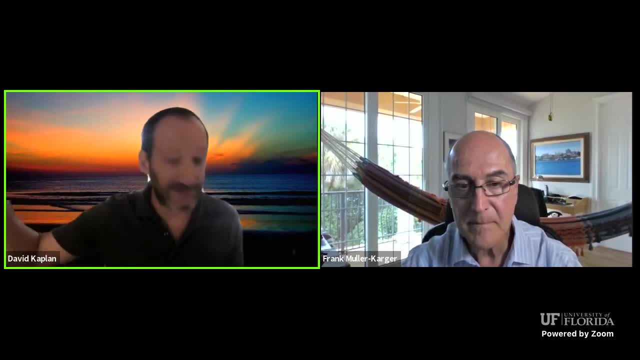 or is the team working to like, yeah, we need to do 75% money on monitoring or whatever it is, but we need a chunk, a big chunk, to do something useful with these data beyond scrapping for grant money after the fact? 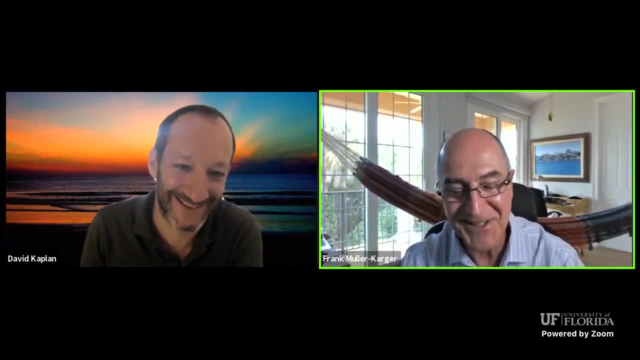 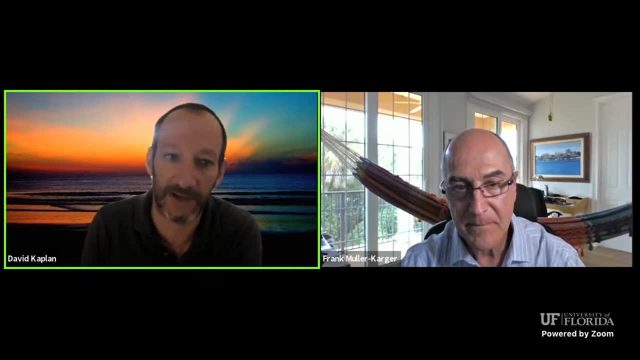 Well, that's our life, isn't it, David? It seems like it, but there's got to be a line here to be. you know, we've got to tap the vein somehow so we can get inference that's useful out of these data. Otherwise, it's a wonderful. 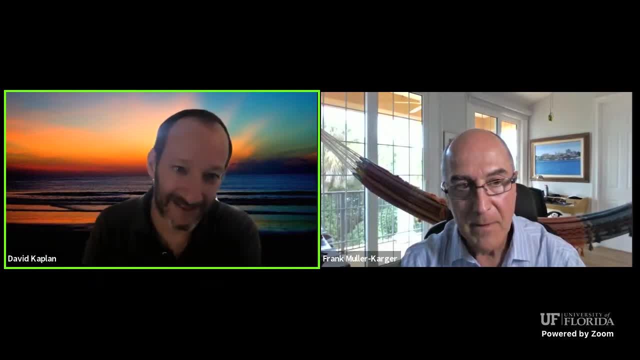 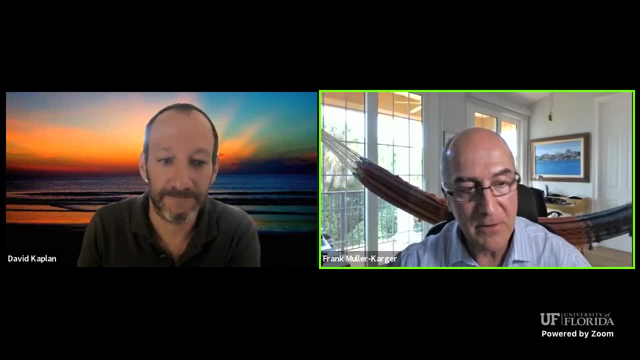 amazing coordinated database of data and that's it. Well, I totally I agree with you And there is no one answer to this. I think that you do work with a user to try to show the need. If the user is one off and one single person, it's not as important. 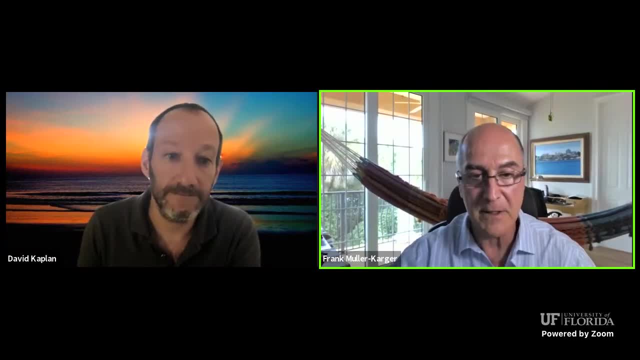 for a government entity or industry to fund the continuing collection and organization of the data. So we work with several groups. in the US The Integrated Ocean Observing System is a critical group that serves as that boundary organization. So in the in the Gulf of Mexico we work with something called GCOOS. 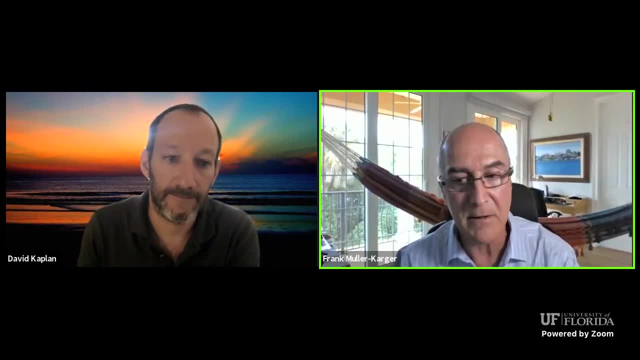 the Gulf of Mexico Coastal Ocean Observing System. And then on the Atlantic side, we work with SECURA, the Southeast Coastal Ocean Regional Association. In the Caribbean, we work with CARICOOS, the Caribbean Coastal Ocean Observing System. And so in the US, 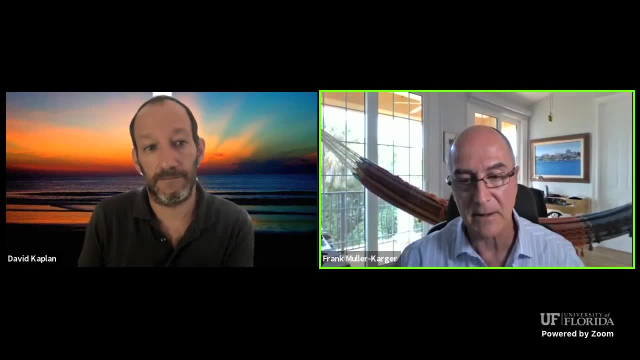 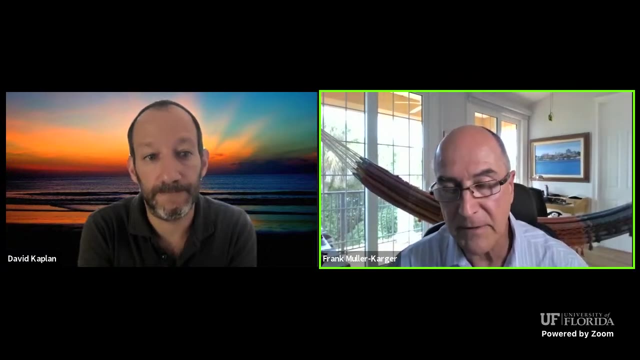 you have these regional associations of IUs that a big part of their job is to connect the user with scientists and vice versa. They're running into the same problem. Their budget is limited, They're always short, They cannot sponsor everything that they want, So we are trying to you know in a way. 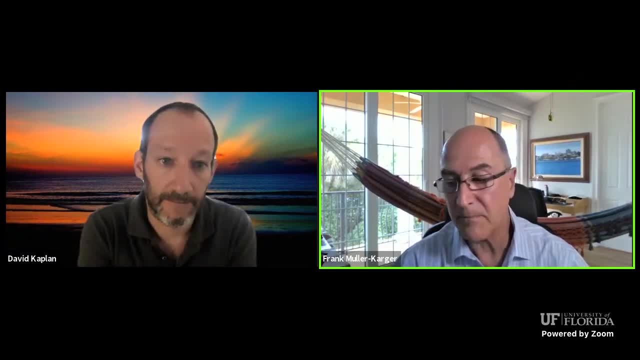 that the decade, the UN decade- is a mechanism to highlight this need of connecting users to observers through science. So it's not. I don't want to minimize the importance of a mechanism like the decade to advertise this requirement for funding, but that's what it is. You know, nothing works without funding, And so you have to organize the. 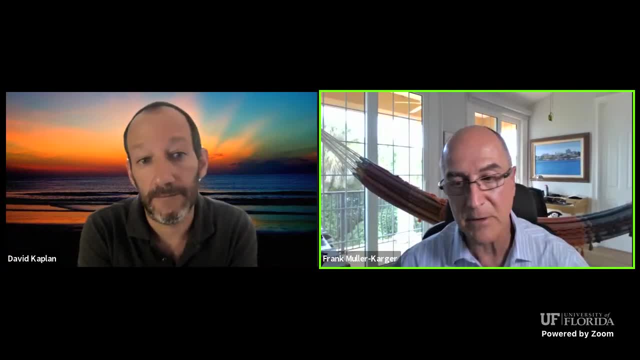 science community better to be relevant to people, not just to ourselves, because I mean, I cannot tell you how many papers I've written that maybe my students read them because I tell them to read it, but that's about it, You know. So what's the point of that? And so if the information that we're producing is not useful to more people, 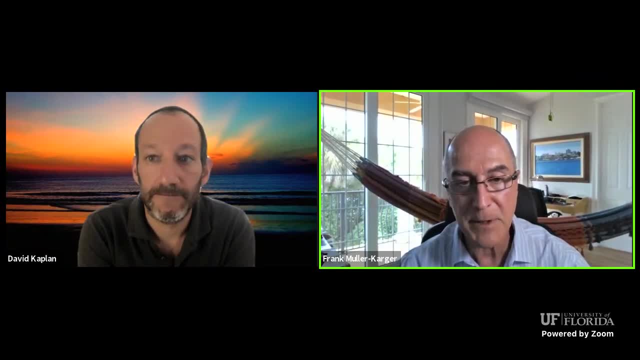 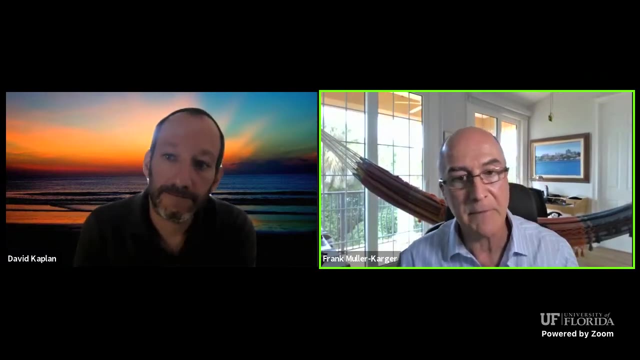 then I think we're wasting a lot of taxpayer money in our own times, And so I think that this is part of the effort is is trying to- yeah, we should do curiosity driven science, because there's many things that we discover that wouldn't come any other way and that have an application. 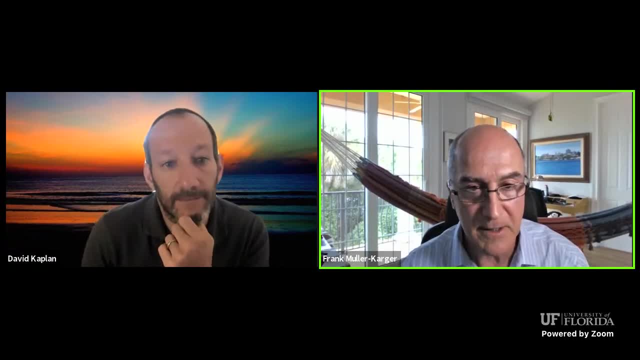 If we didn't look for an aninia, you know, we would have never done that, And that was discovered through science. Right Things like that. Okay, there's untold examples, So you do have to have a hypothesis-driven science. 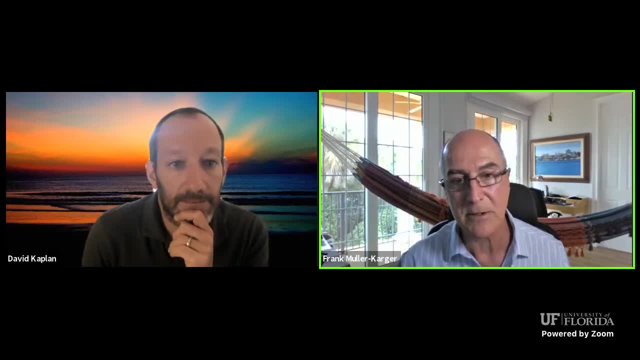 but also you need to do that in a way that is conscious that somebody has to, in the end, use some of the things that you're doing, And ideally you should be aware of societal needs and be in tune. If you ask a manager, what do you need? 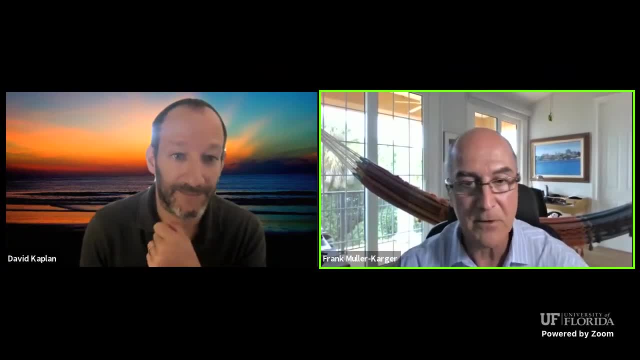 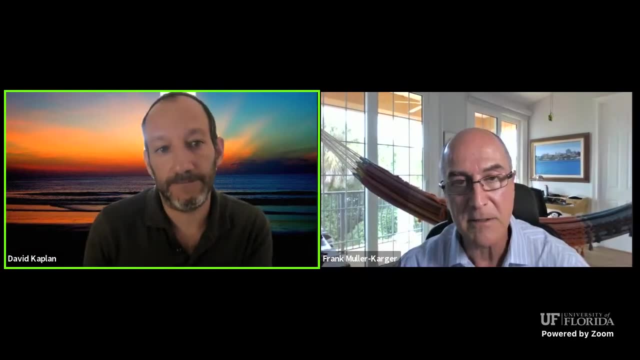 And often, well, I don't know- I mean, what do you have? And you ask each other the same question until you start talking with each other and maybe there's a dialogue that can lead someplace. Well, I think your examples of the portals. 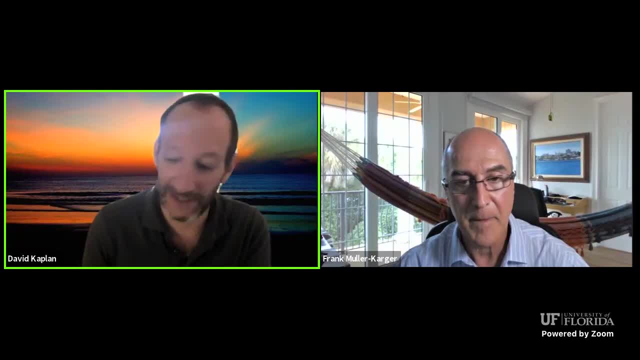 like the early warning systems that you've set up, they were motivated by need. Their potential to be realized came not only from the data but, as you know, the remote sensing algorithm of X or Y. it works or it doesn't work. 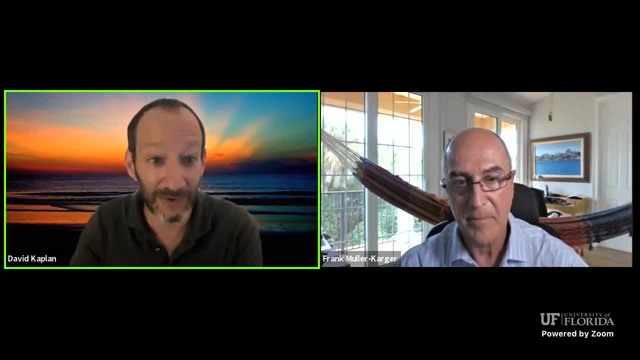 It improves when you work with the stakeholders. So it's not just a stakeholder who says no, it's not working for this purpose And then so it may be targeted to a small set of users, but those are the people on the ground. 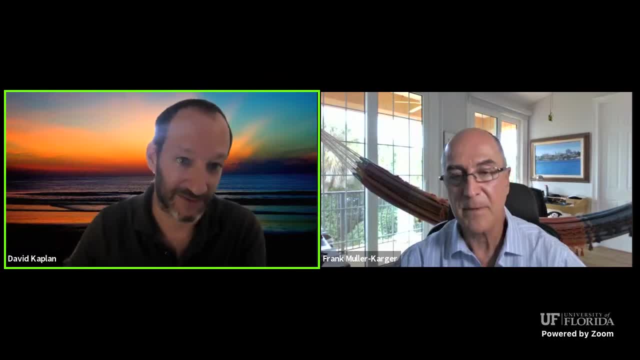 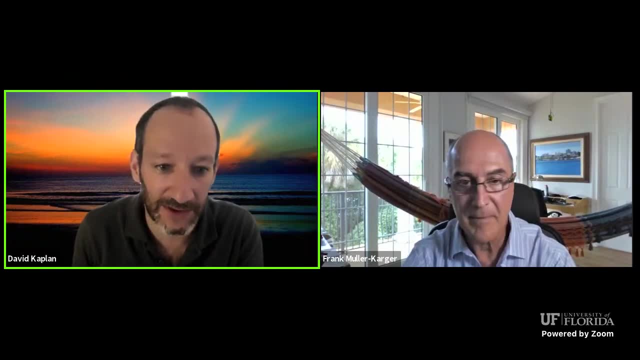 trying to make sense of their observations, sort of, and you're adding to that Any other. so we've heading up. we got about one more minute And Calvin a question, or Liz a question? Hi Frank, It's really nice to see you again here. 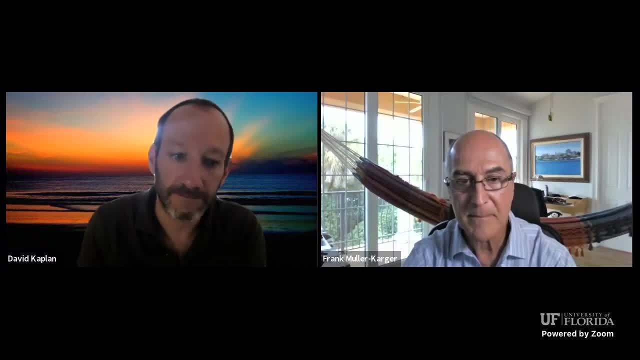 And yeah, I'm just thank you for talking. I'm just really interested in, like you mentioned, how does this kind of different scales of data just kind of could be incorporated or linked, and you guys are kind of working on that. So I'm just wondering, like, what kind of ways that is there available? 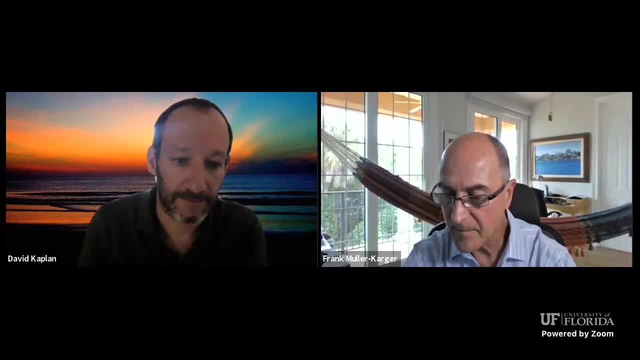 or you know what kind of methodology is there to actually linking, for example, you mentioned genetic biodiversity and socioeconomic data. These are really like wide data sets to be linked, So I'm just wondering how is that Could be done. Yeah, what's the general approach. 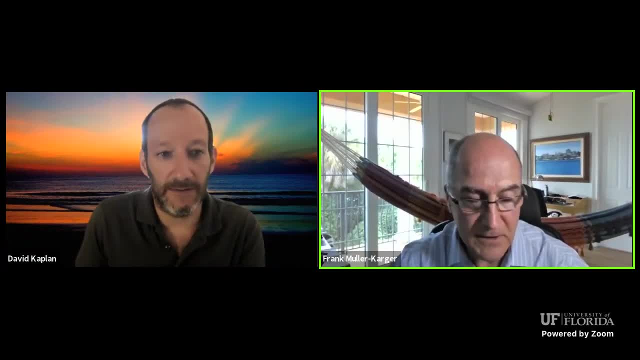 Yeah, with omics data there's, it's actually a very active field of research. There's two ways that people use eDNA data right now. One is you can use primers or markers for genes that you know is something that you want to detect. 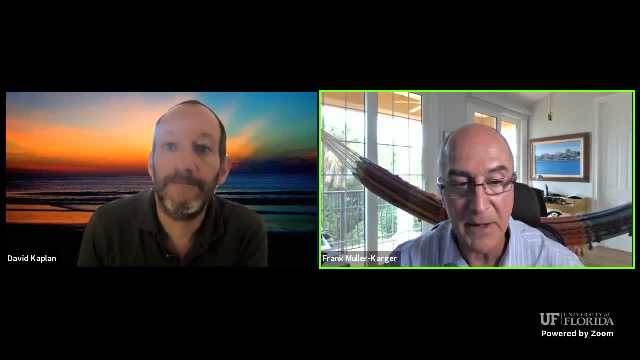 if you want to detect a specific species, like an invasive species, And so this is actually operational. Many groups use it. Yeah, Many agencies use it. It is very well-established science. What is not so established is the discovery of what's there. 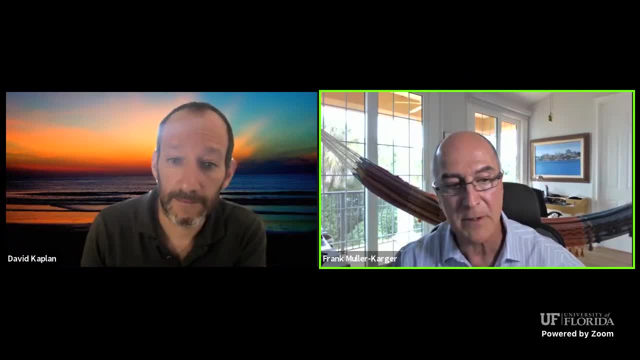 just by looking at everything, You know you can use several different primers. You collect a glass of water and you try to see what's there And there's a lot of questions about you know how long that eDNA is viable for. 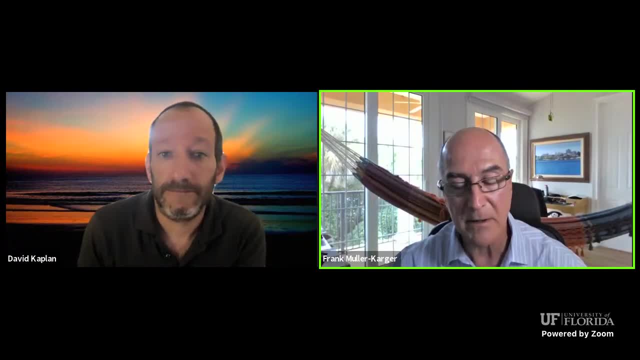 Did you get a big chunk of a whale in your sample and that contaminates and overwhelms everything? Or what do you do with all these taxa that you don't find in any database and they just don't look like anything? And so you have all these, you know. 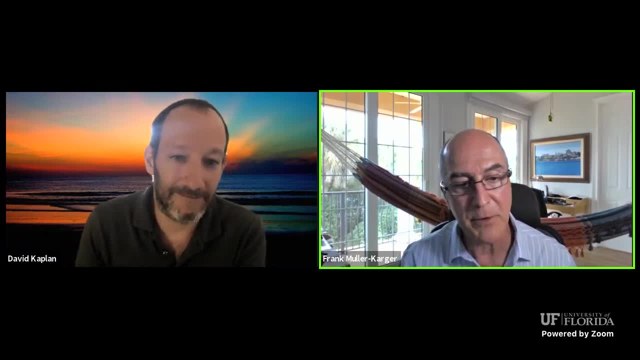 half of your sample could be dark taxa. So a lot of people are now involved in trying to understand what is it that you can do with this enormous explosion in omics, methods and data. Another problem is that every lab you go to does things differently. 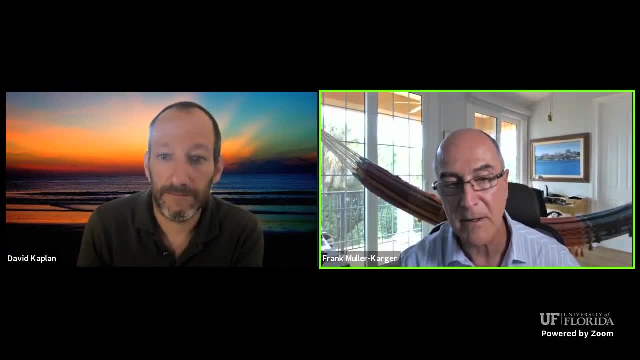 So the eDNA data or the omics data that you collect and one group may do at your university is different from what I collect, and so they're not comparable. So how do we get to the point where people are collecting data and processing it in a way that is more or less standardized? 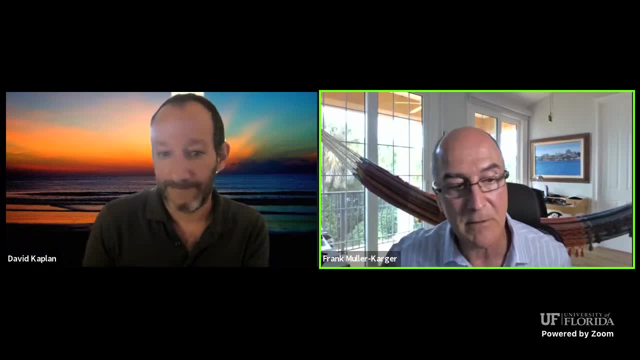 as you're going through a technological revolution And we're not there yet. so I don't think that we have an answer on exactly how do you combine, for example, the omics data with everything else. We know how to combine, for example. 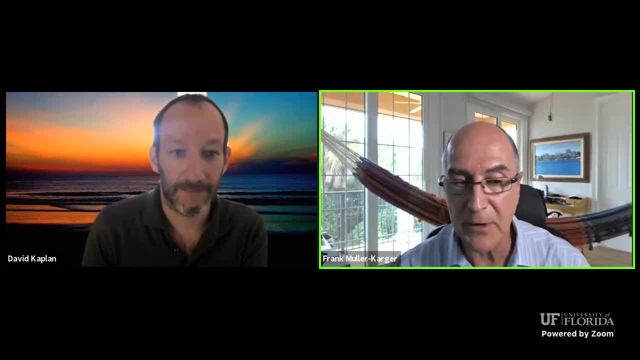 the abundance of organisms or productivity with temperature, and even have some very primitive models that say, well, if your temperature goes up, the physiology or the productivity of something may go up until a point and then things don't go up anymore. But in order to get there you have to have the data.